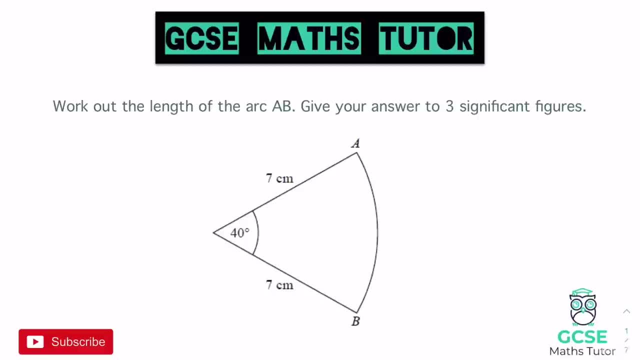 looking at normal sectors here, and this particular question is asking us to look at the length of the arc, and then we're also going to have a look at working out the area of one of these. so do grab a piece of paper, grab a pen, make some notes, and we're going to have a look at this question to 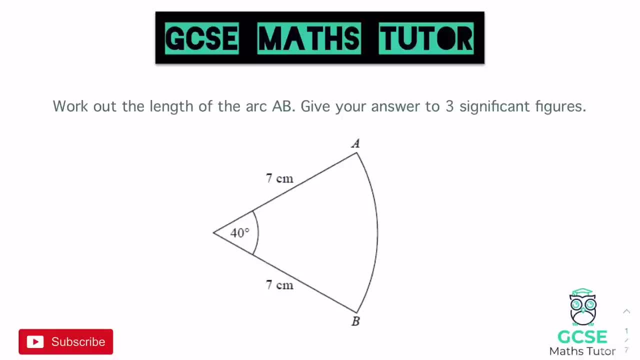 start with. So it says: work out the length of the arc AB. so from A to B, is this arc right here? and that's what we're going to work out. Now, when we're looking at the length of the arc, we're looking at part of the circumference and the formula for the circumference is: circumference equals the diameter. 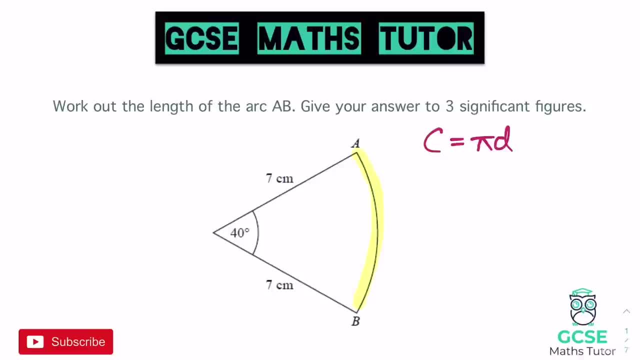 times pi or pi times diameter. okay, so that's all we're going to do. we're just going to do pi times diameter, but then we're going to look at it as a fraction of the whole circle here, because obviously this is only part of a circle and we're going to have a look at what fraction it is. Now the key. 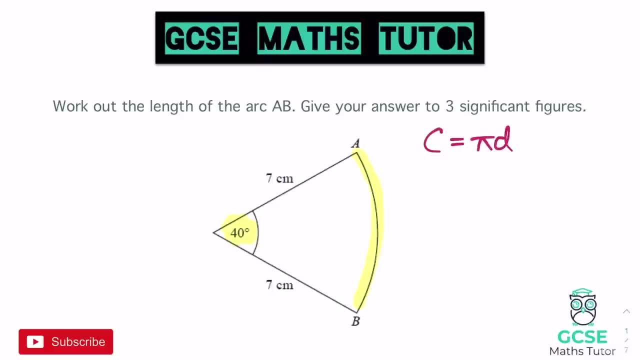 is this angle right here. so we've got 40 degrees at the moment and we know that in a circle there are 360 degrees. so the fraction of the circle that we're looking at here is 40 out of 360. okay, and that's what fraction of the full circle we're looking at. So, in terms of the length of the arc, 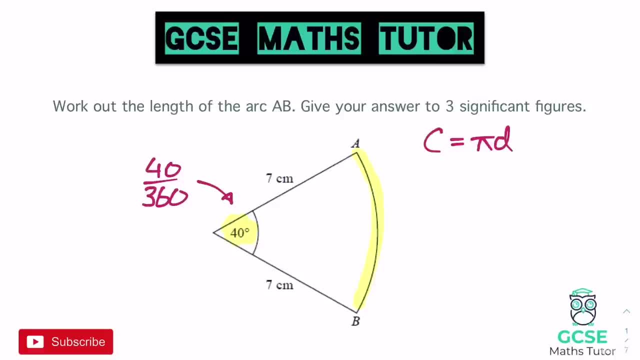 that is the fraction of the circumference that we're actually going to be finding. okay, we're going to be finding 40 over 360- lots of the circumference, okay, and we could go about simplifying that if we wanted to, but we're going to do this all on the calculator, so there's no need for us to. 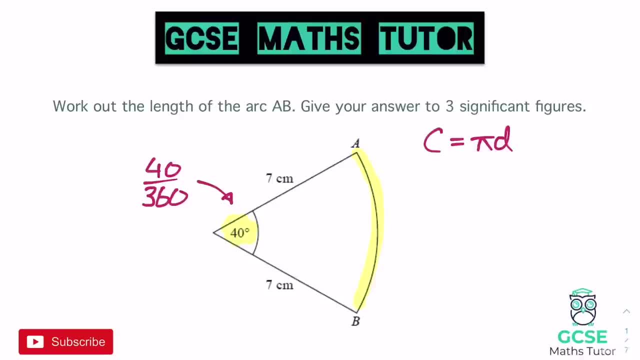 be simplifying these fractions. So to work out the full circumference, I first need to know what the diameter is. now, this particular question, as it's a sector, tells us the radius. okay, it says the radius there, which is 7, and the diameter is double that. okay, so we're going to double that for the diameter, so the 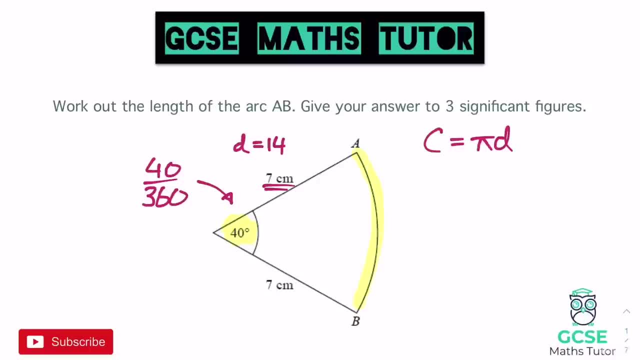 diameter is going to be 14.. So to work out the full circumference, I would do pi and I would times that by 14. okay, and if I work that out on the calculator, let's have a look what it comes out. as pi times 14 comes out as 43.982.. Now that's fine. that's the full circumference, but I only want part. 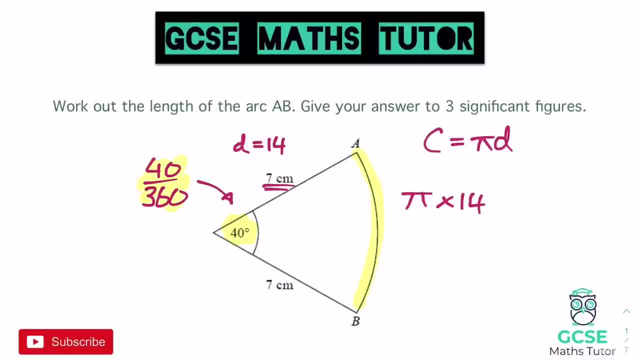 of it and I've already established that it's 40 over 360.. So straight away on the calculator, rather than working that out, I'm just going to straight away. I'm just going to times that by the fraction that we're looking for, which is 40 over 360.. There we go. so if I type that in, so pi times 14 times. 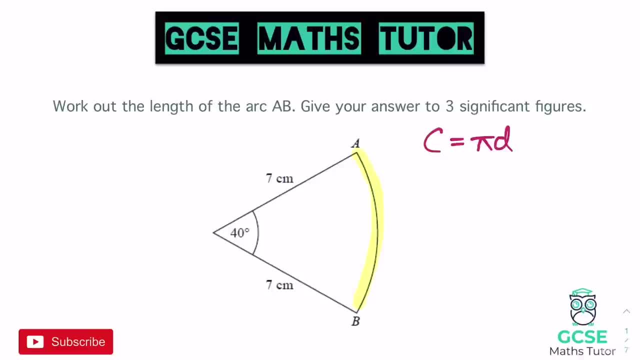 times pi or pi times diameter. okay, so that's all we're going to do. we're just going to do pi times diameter, but then we're going to look at it as a fraction of the whole circle here, because obviously this is only part of a circle and we're going to have a look at what fraction it is. Now the key. 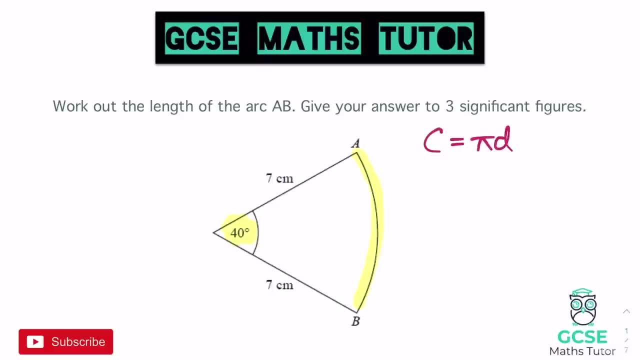 is this angle right here. so we've got 40 degrees at the moment and we know that in a circle there are 360 degrees. so the fraction of the circle that we're looking at here is 40 out of 360. okay, and that's what fraction of the full circle we're looking at. So, in terms of the length of the arc, 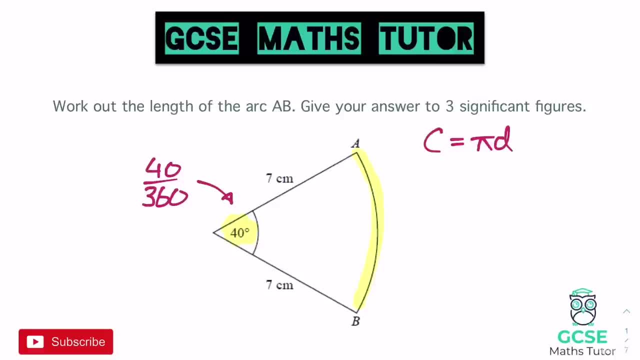 that is the fraction of the circumference that we're actually going to be finding. okay, we're going to be finding 40 over 360- lots of the circumference, okay, and we could go about simplifying that if we wanted to, but we're going to do this all on the calculator, so there's no need for us to. 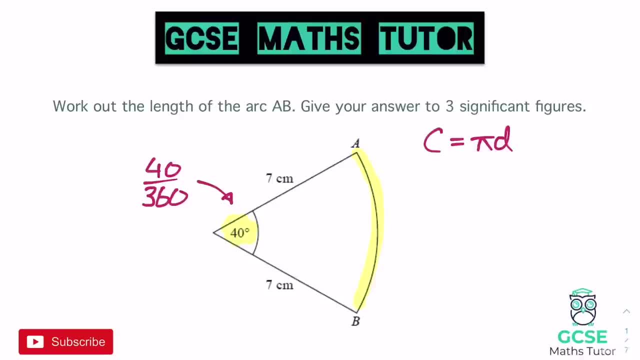 be simplifying these fractions. So to work out the full circumference, I first need to know what the diameter is. now, this particular question, as it's a sector, tells us the radius. okay, it says the radius there, which is 7, and the diameter is double that. okay, so we're going to double that for the diameter, so the 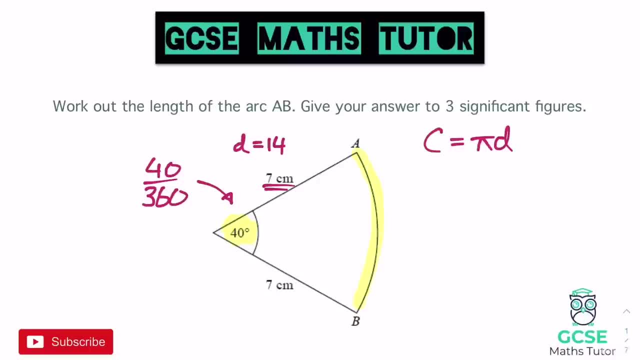 diameter is going to be 14.. So to work out the full circumference, I would do pi and I would times that by 14. okay, and if I work that out on the calculator, let's have a look what it comes out. as pi times 14 comes out as 43.982.. Now that's fine. that's the full circumference, but I only want part. 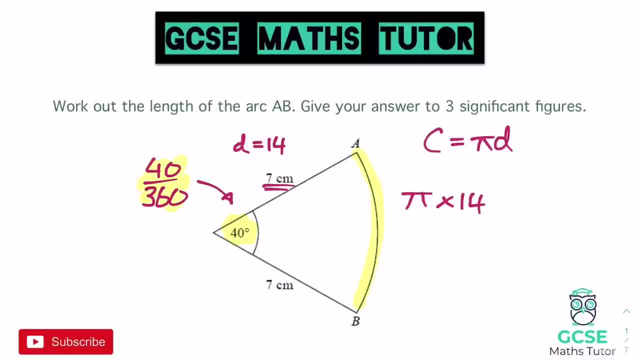 of it and I've already established that it's 40 over 360.. So straight away on the calculator, rather than working that out, I'm just going to straight away. I'm just going to times that by the fraction that we're looking for, which is 40 over 360.. There we go. so if I type that in, so pi times 14 times. 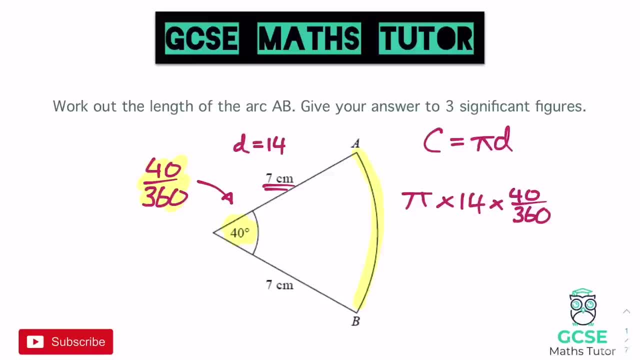 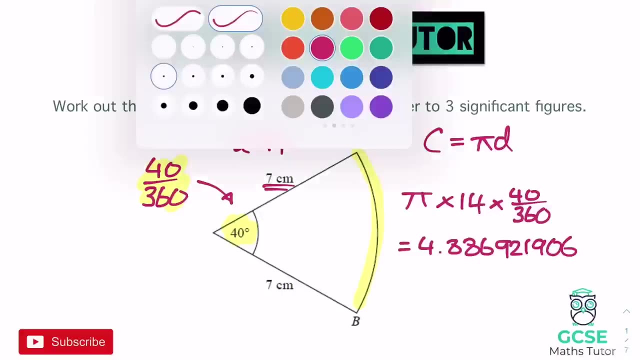 40 over 360 and I get my final answer there and that comes out as 4.886921906.. There we go and we'll write all those numbers down. Now. obviously it says in this question and it'll always tell you a specific way to round it. 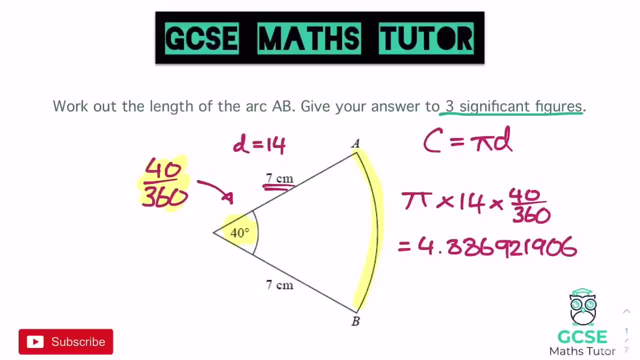 and here it says three significant figures. so if we round that to three significant figures, then so 4,, 8,, 8, chop it after the 8,, there we are: it's a 6 afterwards. so that's going to round that final 8 up there. so that is going to be a final answer of 4.89.. There we go and just have a look. 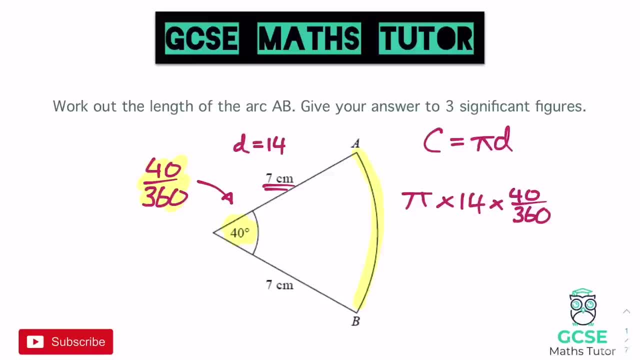 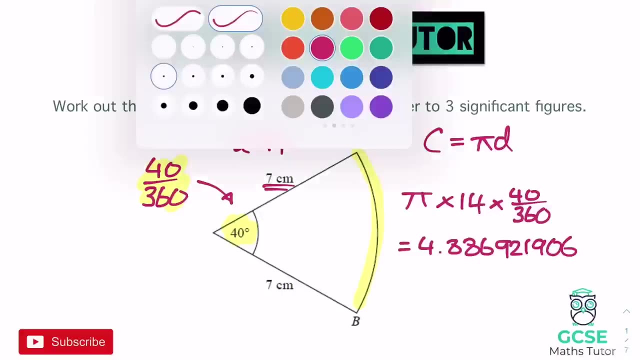 40 over 360 and I get my final answer there and that comes out as 4.886921906.. There we go and we'll write all those numbers down. Now. obviously it says in this question and it'll always tell you a specific way to round it. 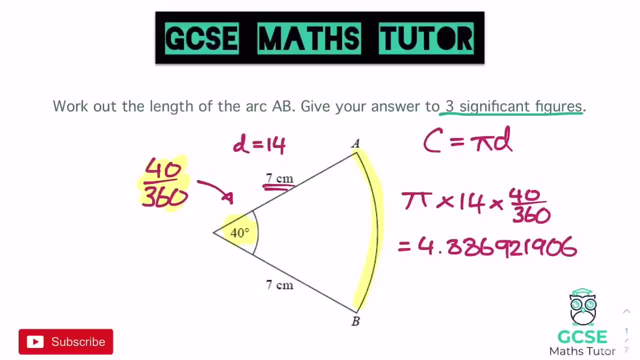 and here it says three significant figures. so if we round that to three significant figures, then so 4,, 8,, 8, chop it after the 8,, there we are: it's a 6 afterwards. so that's going to round that final 8 up there. so that is going to be a final answer of 4.89.. There we go and just have a look. 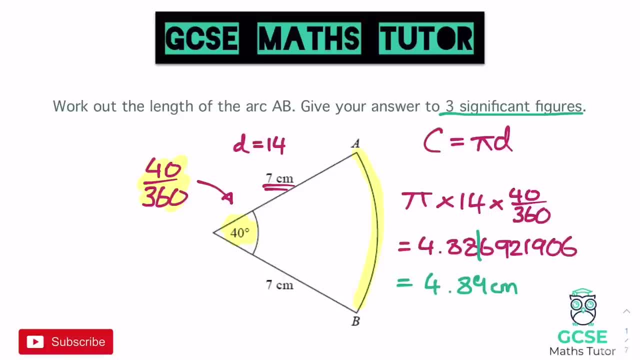 in the question it's centimetres, so that's 4.89 centimetres. and there we go. that's our final answer. So all you've got to do is obviously have a good understanding of the formula. so circumference is pi times diameter, and then obviously you've got to have a good understanding. 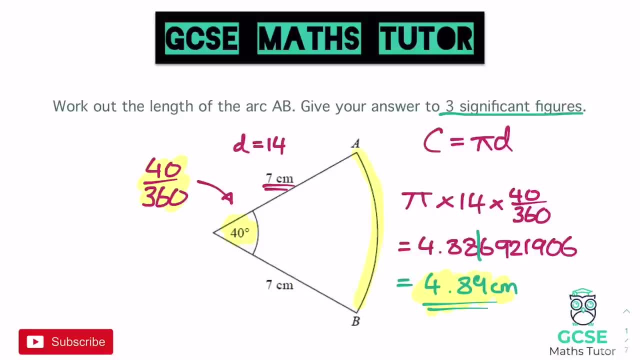 of what fraction of the circle you've actually got in front of you when you're looking at one of these sectors. So there we go. what we did was circumference is pi times diameter, multiplied it by 40 over 360, and that gave us the length of the arc. Now a question like this might also ask: 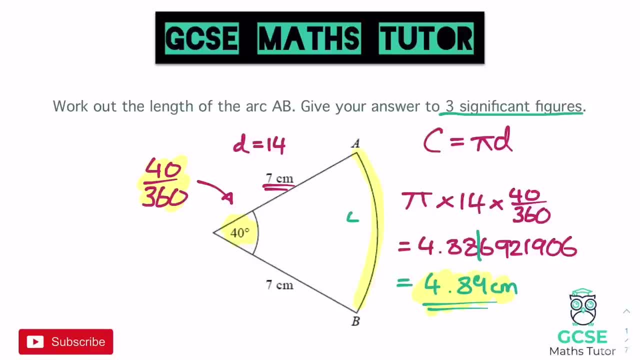 you to find the perimeter. so at the moment we've established that this length here is 4.89. but if it did ask us to find the perimeter, that would be the full length all the way around. So the yellow line I've highlighted is 4.89, but then we also have these two lengths here, which are both 7 and 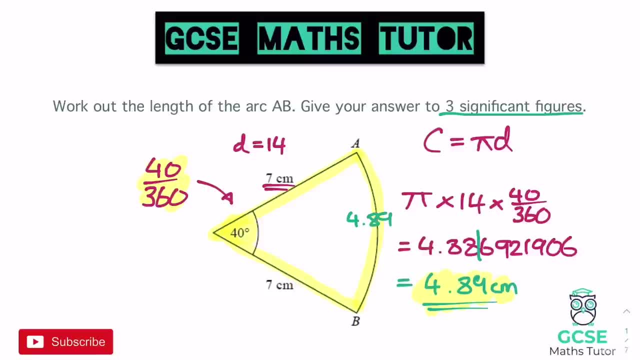 we would add them up to 4.89.. So that's 4.89, and then we also have these two lengths here which are all together to get the perimeter there. So 7 plus 7 is 14 plus the 4.89 and come out as 18.89. for 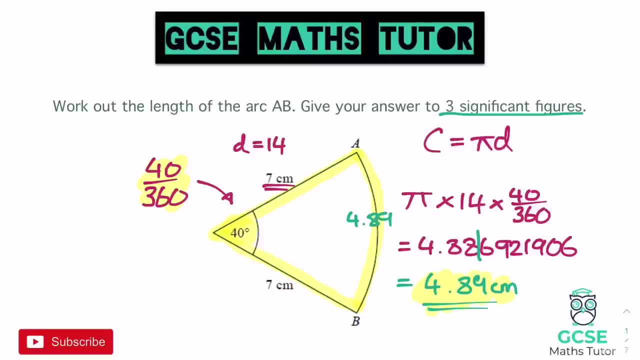 the full perimeter. But again, this question was only asking for the length of the arc, but just thinking about different things that you could actually be asked to find on a particular question like this. Right, okay, so we're going to have a look at working out the area of a sector. 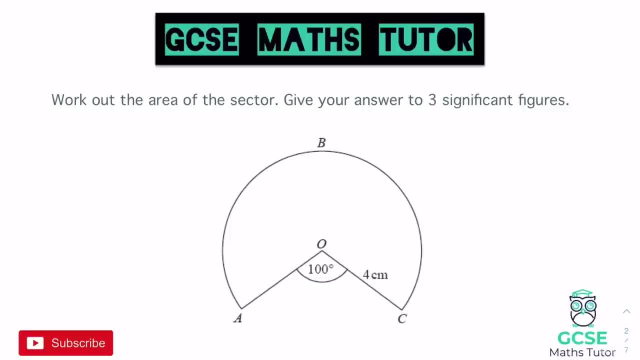 Okay. so once you've obviously got to grips with that previous question, looking at the length of the arc, working out the area of a sector isn't really any more complicated. okay, because the area of a circle, which we'll write down here, is pi times the radius squared, or pi r squared. Now, when it comes to this sort of question, 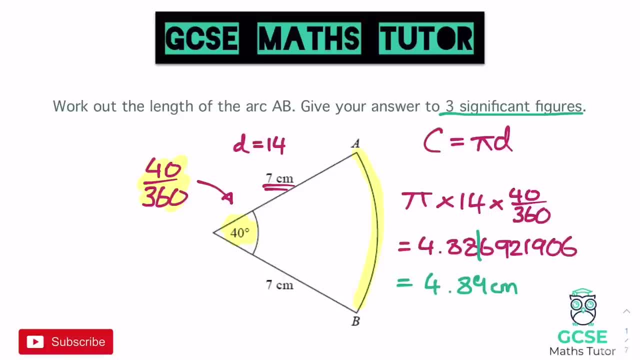 in the question it's centimetres, so that's 4.89 centimetres. and there we go. that's our final answer. So all you've got to do is obviously have a good understanding of the formula. so circumference is pi times diameter, and then obviously you've got to have a good understanding. 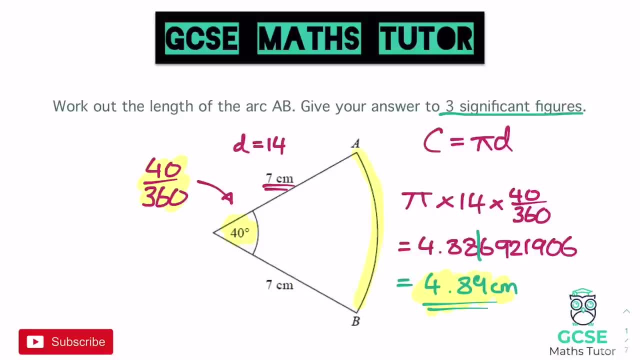 of what fraction of the circle you've actually got in front of you when you're looking at one of these sectors. So there we go. what we did was circumference is pi times diameter, multiplied it by 40 over 360, and that gave us the length of the arc. Now a question like this might also ask: 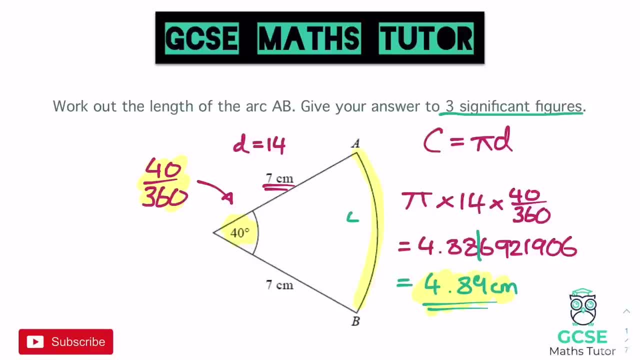 you to find the perimeter. so at the moment we've established that this length here is 4.89. but if it did ask us to find the perimeter, that would be the full length all the way around. So the yellow line I've highlighted is 4.89, but then we also have these two lengths here, which are both 7 and 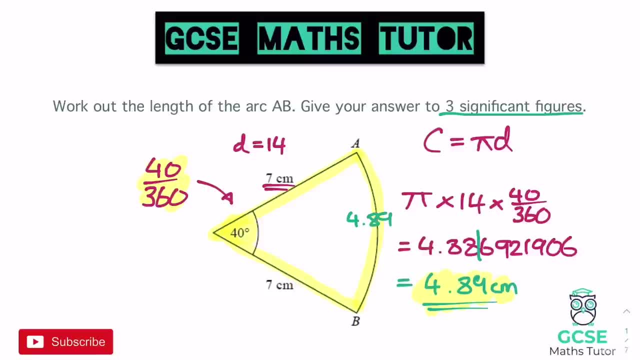 we would add them up to 4.89.. So that's 4.89, and then we also have these two lengths here which are all together to get the perimeter there. So 7 plus 7 is 14 plus the 4.89 and come out as 18.89. for 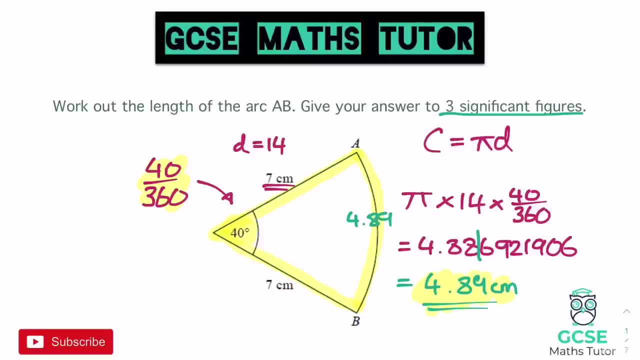 the full perimeter. But again, this question was only asking for the length of the arc, but just thinking about different things that you could actually be asked to find on a particular question like this. Right, okay, so we're going to have a look at working out the area of a sector. 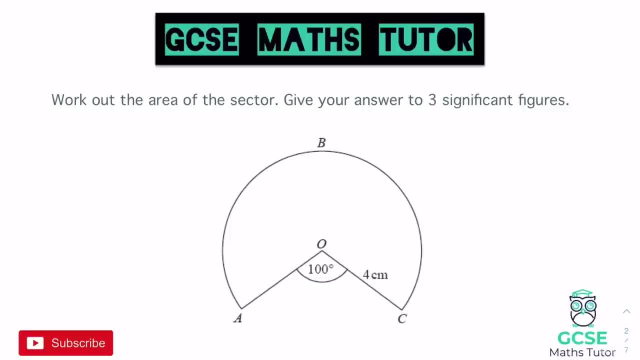 Okay. so once you've obviously got to grips with that previous question, looking at the length of the arc, working out the area of a sector isn't really any more complicated. okay, because the area of a circle, which we'll write down here, is pi times the radius squared, or pi r squared. Now, when it comes to this sort of question, 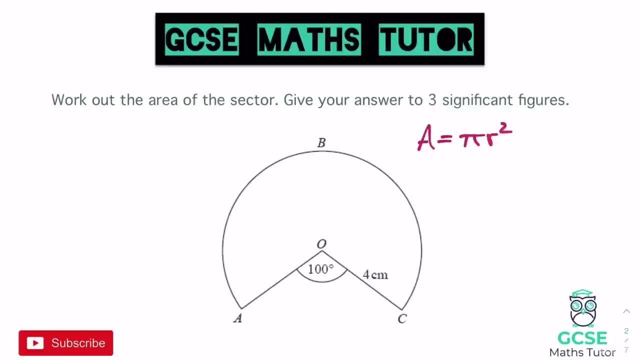 obviously we just need to make sure that we are establishing what fraction of the circle it is. again, and this is a major sector, here we've got quite a large sector obviously, obviously thinking about the size of the full circle, and we've got a little sector there that's been chopped off. but 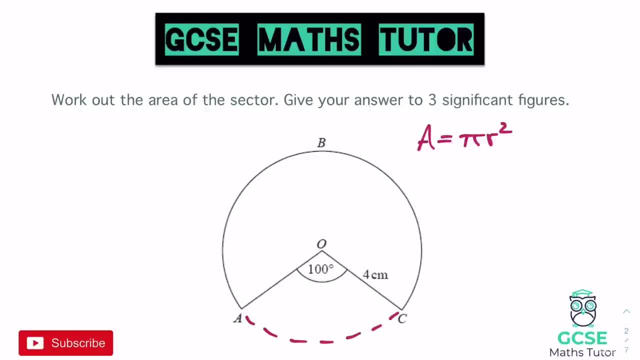 we've got quite a big sector that we're actually working out, the area of. Okay. so the actual sector we're looking at the angle for that is on the other side, just here. so we're going to have to take that 100 away from 360 to establish what's left, and that is 260 degrees. Okay, so that's the. 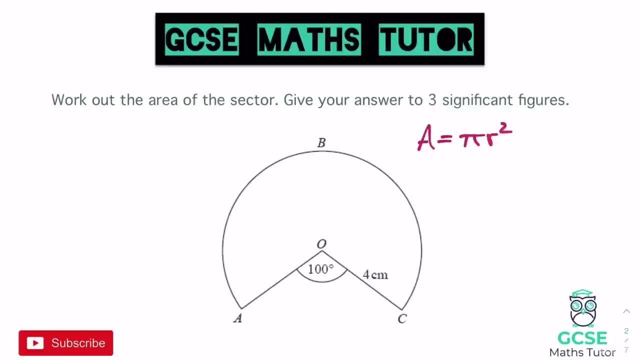 obviously we just need to make sure that we are establishing what fraction of the circle it is. again, and this is a major sector, here we've got quite a large sector obviously, obviously thinking about the size of the full circle, and we've got a little sector there that's been chopped off. but 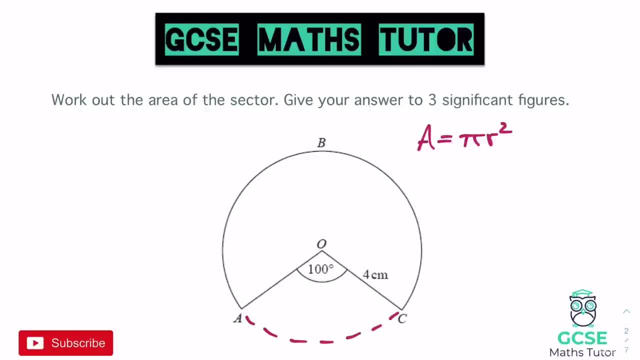 we've got quite a big sector that we're actually working out, the area of. Okay. so the actual sector we're looking at the angle for that is on the other side, just here. so we're going to have to take that 100 away from 360 to establish what's left, and that is 260 degrees. Okay, so that's the. 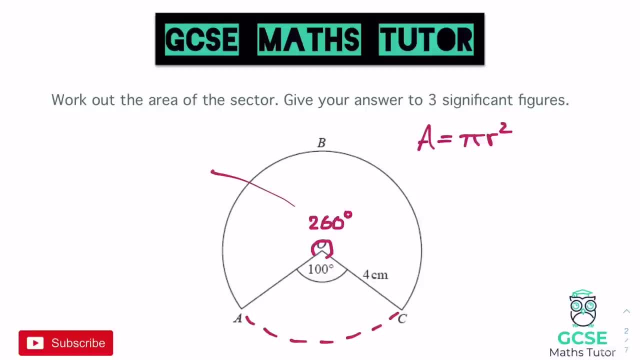 fraction of the circle. we're looking at 260 out of 360 and let's just label that so we know that. so that's 260 out of 360. So we're going to follow the same process. obviously, this time it says work out the area of the sector. so we're going to do pi times the radius squared, the radius down there. 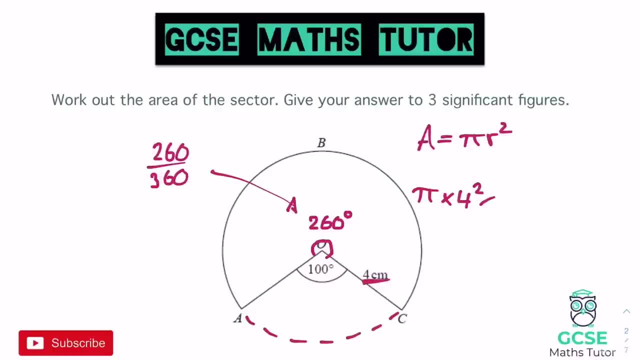 four, so times four squared, and then again just times by the fraction that we're looking at, which is 260.. 260 over 360 and typing that into the calculator, pi times four squared times, and let's just type that in 260 over 360 and that gives me a final answer here of 36.3028- quite a lot of decimals. 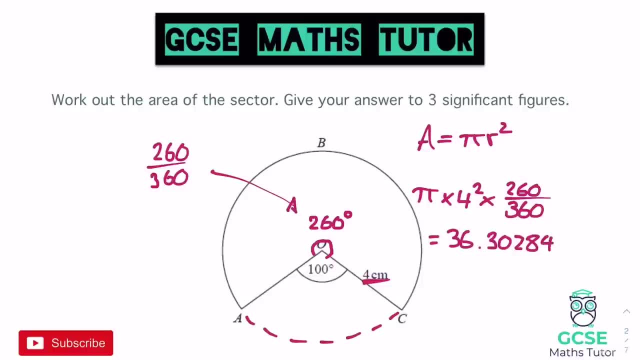 here: 30284844. there we go, and again we're going to round this to three significant figures, as it says up here. so let's round that off: So 363. chop it up to the three, it's a zero there, so that's going to stay the same. so we've got 36.3. 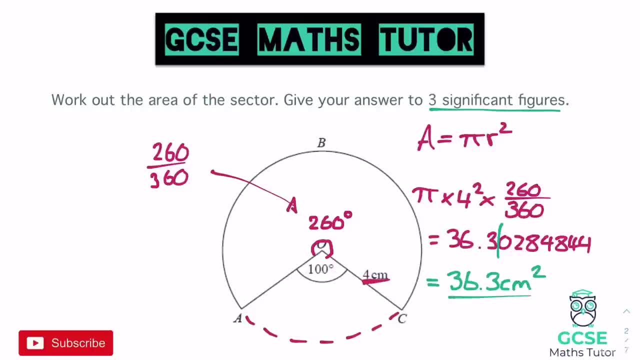 and that is centimeters squared. there we go. obviously, for an area, we need to make sure we get the right units in there. so 36.3 centimeter squared is our final answer. So there we go. that's all you need to do, obviously. you just need to know those two formulas, whether you ask for the 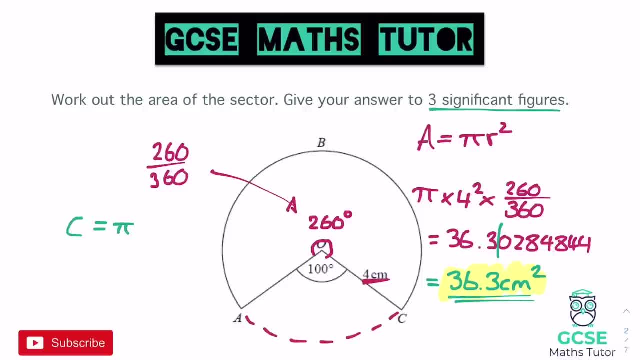 circumference, which is where you're going to do pi times diameter. or if you ask for the area and we're going to do pi times the radius squared, okay, Now, both of those. we're obviously going to multiply that by whatever fraction we're looking at. so when it comes to the sector here, we'll call that angle x over 360, and the same for the one. 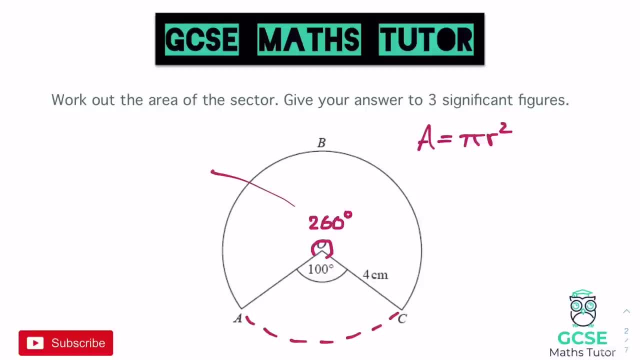 fraction of the circle. we're looking at 260 out of 360 and let's just label that so we know that. so that's 260 out of 360. So we're going to follow the same process. obviously, this time it says work out the area of the sector. so we're going to do pi times the radius squared, the radius down there. 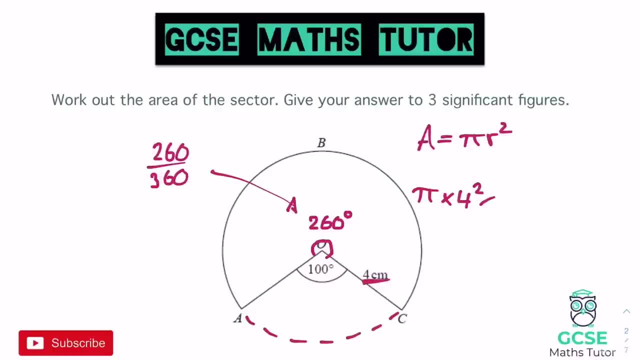 four, so times four squared, and then again just times by the fraction that we're looking at, which is 260.. 260 over 360 and typing that into the calculator, pi times four squared times, and let's just type that in 260 over 360 and that gives me a final answer here of 36.3028- quite a lot of decimals. 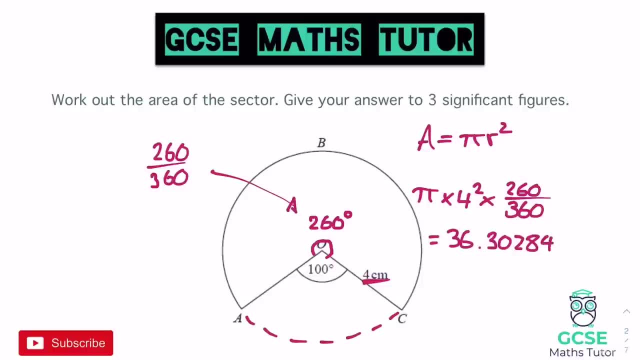 here: 30284844. there we go, and again we're going to round this to three significant figures, as it says up here. so let's round that off: So 363. chop it up to the three, it's a zero there, so that's going to stay the same. so we've got 36.3. 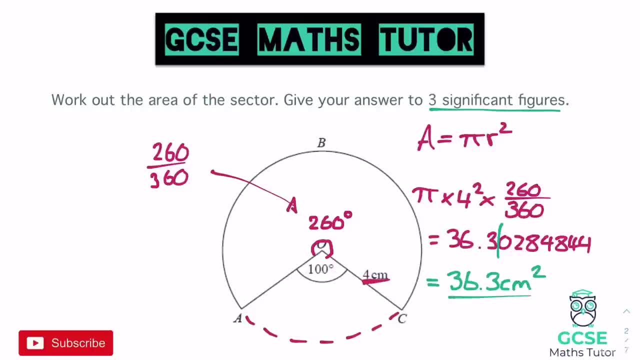 and that is centimeters squared. there we go. obviously, for an area, we need to make sure we get the right units in there. so 36.3 centimeter squared is our final answer. So there we go. that's all you need to do, obviously. you just need to know those two formulas, whether you ask for the 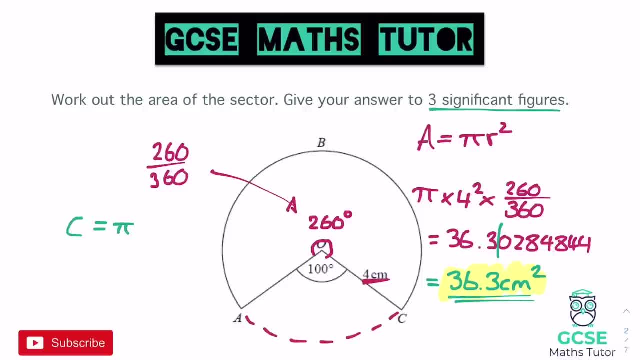 circumference, which is where you're going to do pi times diameter. or if you ask for the area and we're going to do pi times the radius squared, okay, Now, both of those. we're obviously going to multiply that by whatever fraction we're looking at. so when it comes to the sector here, we'll call that angle x over 360, and the same for the one. 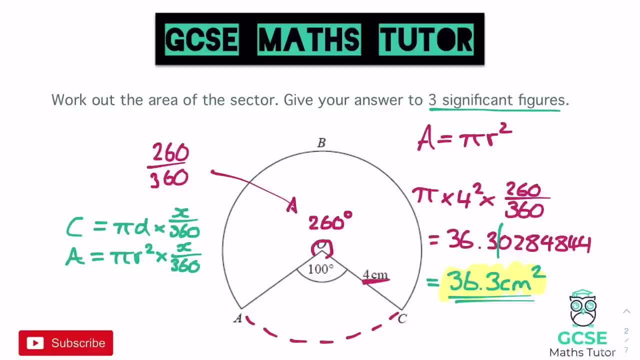 below. there we go, but that circumference and area formula are key to remember, and then, obviously, just thinking about what fraction of the circle it is that we're going to multiply it by Okay, so there we go. that's how we're going to work some of these out now. I've got a couple of questions. 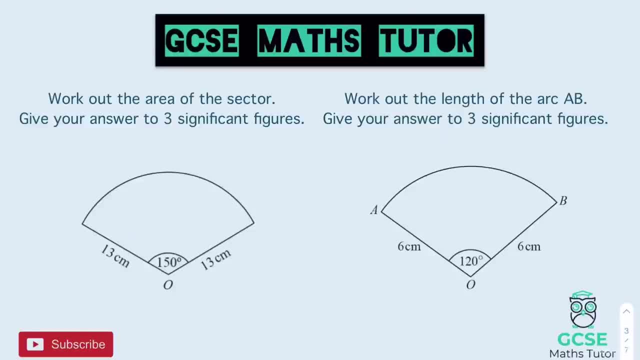 for you to have a go at. Okay, so there's two questions here: one on the left- work out the area of the sector. and one on the right- work out the area of the sector. and one on the right- work out the length of the arc. So have a go at these two questions. pause the video there. I'll go over the. 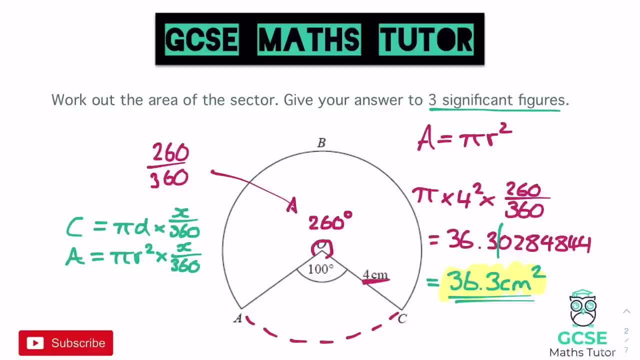 below. there we go, but that circumference and area formula are key to remember, and then, obviously, just thinking about what fraction of the circle it is that we're going to multiply it by Okay, so there we go. that's how we're going to work some of these out now. I've got a couple of questions. 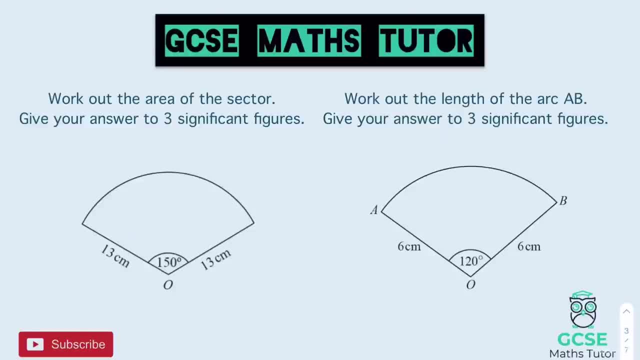 for you to have a go at. Okay, so there's two questions here: one on the left- work out the area of the sector. and one on the right- work out the area of the sector. and one on the right- work out the length of the arc. So have a go at these two questions. pause the video there. I'll go over the. 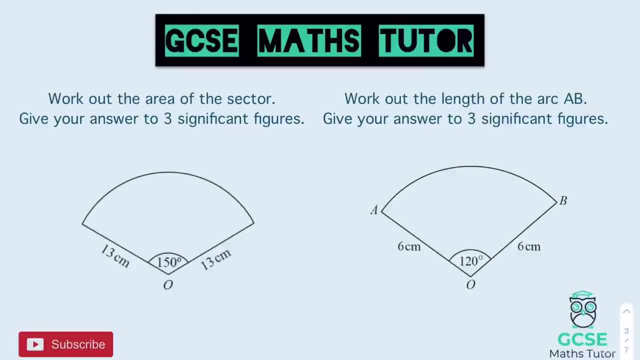 answer in a sec. Okay, so for the first one then. so work out the area of the sector. so we're going to use pi r squared. I'm just going to write that down. there. we go pi r squared and we are obviously working out this fraction of the sector: 150 over 360.. So if we put all the values in, we've got pi. 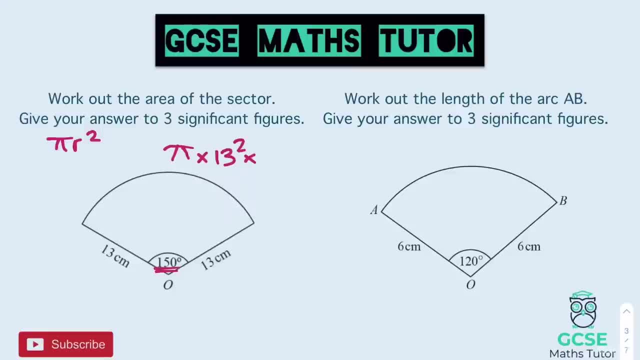 times 13 squared, and then that's going to be times 150 over 360, and that's the fraction that we've got for this one. So we're going to be typing that in pi: times 13 squared, times 150 over 360, and that comes out as: 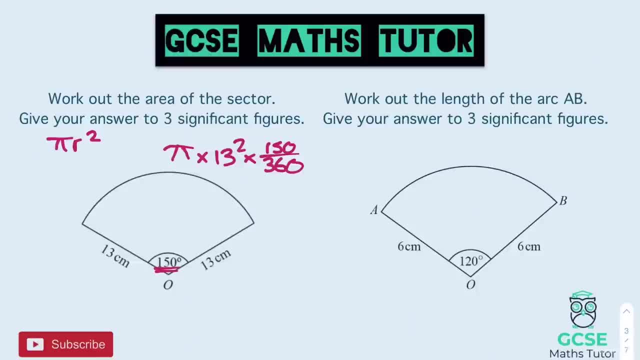 221. let's have a look. let's write this down: 221.22, and there are a few more decimals, but it asks me to round it to three significant figures, which means I'm going to end up chopping that after the one there, so that comes out as a nice whole number 221. it's in centimetres and it's an. 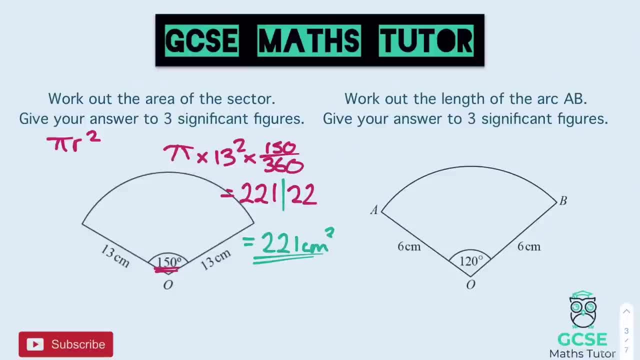 area. so centimetre squared, there we go. so 221 centimetre squared is our final answer. onto the next one, we're now looking at the length of the arc. so again we're working out part of the circumference, this bit here. so we're going to use pi times diameter. okay there. 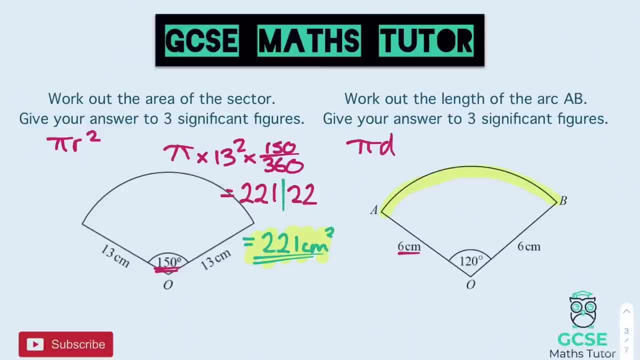 we are. so plug in all these numbers in then. now let's just check out the radius. that's six, so the radius of the diameter is going to be 12. okay, so let's put that all in. we've got pi times 12 times the fraction, this time, which is 120 over 360, and let's see what that gives us. 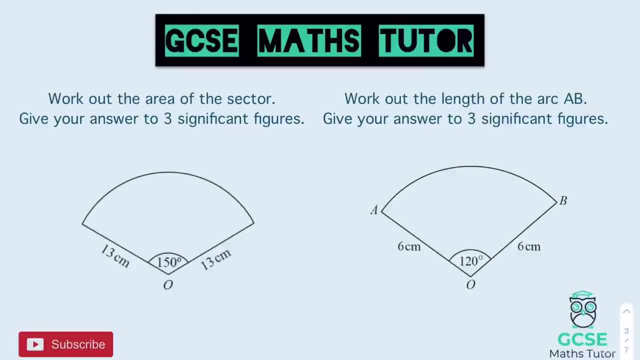 answer in a sec. Okay, so for the first one then. so work out the area of the sector. so we're going to use pi r squared. I'm just going to write that down. there. we go pi r squared and we are obviously working out this fraction of the sector: 150 over 360.. So if we put all the values in, we've got pi. 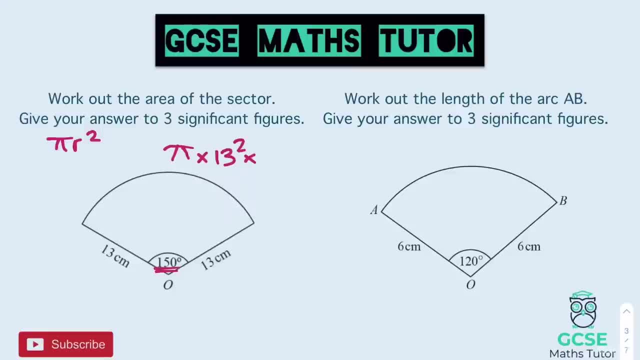 times 13 squared, and then that's going to be times 150 over 360, and that's the fraction that we've got for this one. So we're going to be typing that in pi: times 13 squared, times 150 over 360, and that comes out as: 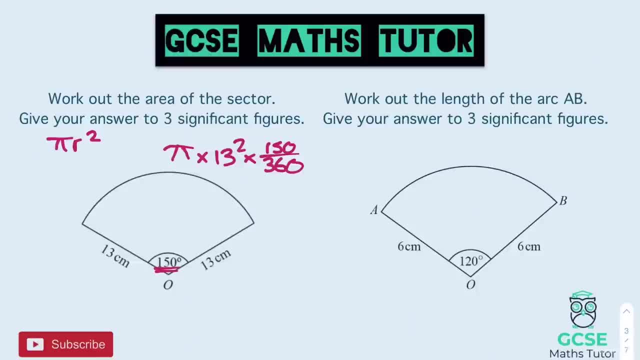 221. let's have a look. let's write this down: 221.22, and there are a few more decimals, but it asks me to round it to three significant figures, which means I'm going to end up chopping that after the one there, so that comes out as a nice whole number 221. it's in centimetres and it's an. 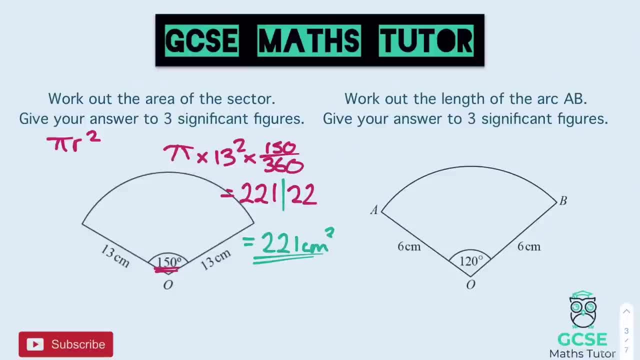 area. so centimetre squared, there we go. so 221 centimetre squared is our final answer. onto the next one, we're now looking at the length of the arc. so again we're working out part of the circumference, this bit here. so we're going to use pi times diameter. okay there. 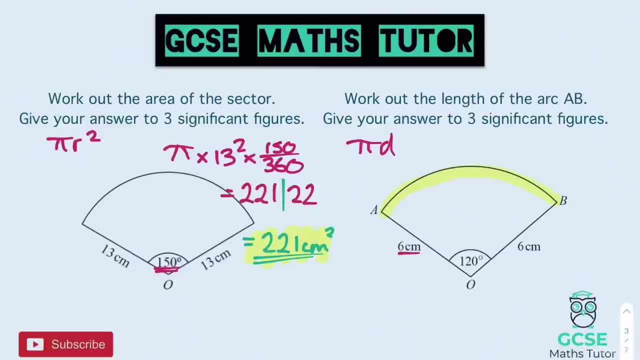 we are. so plug in all these numbers in then. now let's just check out the radius. that's six, so the radius of the diameter is going to be 12. okay, so let's put that all in. we've got pi times 12 times the fraction, this time, which is 120 over 360, and let's see what that gives us. 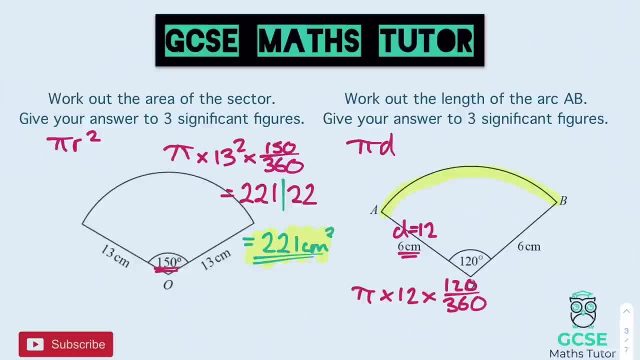 pi times 12, times 120 over 360, and that gives us a final answer here of 12.566, with a few more decimals, but again it's three significant figures, so I'm going to leave it there. chop it after the five and that is going to become 12.6, and its units are centimetres. there we go, so 12.6 centimetres. 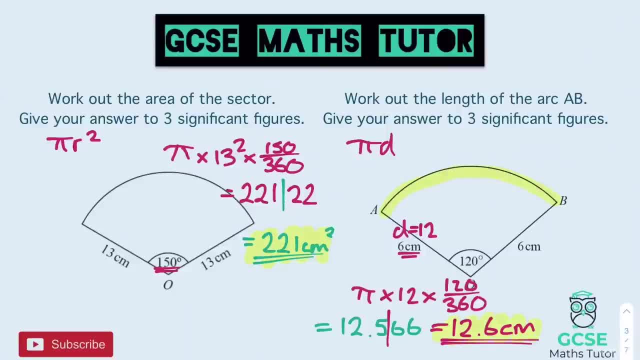 and there's our final answer for the second question, right, okay, let's have a look at some slightly different then applying, obviously, some of these rules, maybe a little bit in reverse as well. so let's have a look at one of those, okay, so this question says the sector has a perimeter of 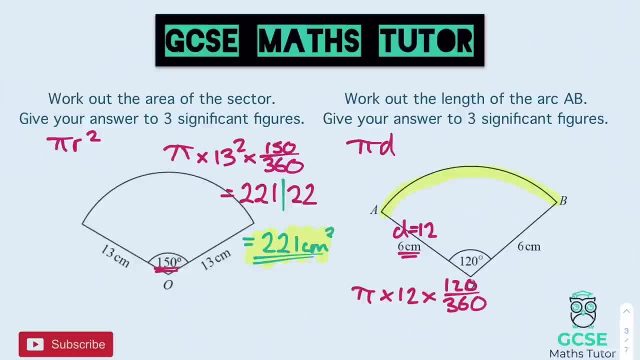 pi times 12, times 120 over 360, and that gives us a final answer here of 12.566, with a few more decimals, but again it's three significant figures, so I'm going to leave it there. chop it after the five and that is going to become 12.6, and its units are centimetres. there we go, so 12.6 centimetres. 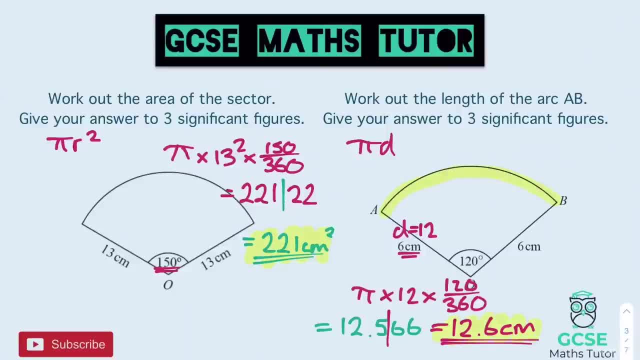 and there's our final answer for the second question, right, okay, let's have a look at some slightly different then applying, obviously, some of these rules, maybe a little bit in reverse as well. so let's have a look at one of those, okay, so this question says the sector has a perimeter of 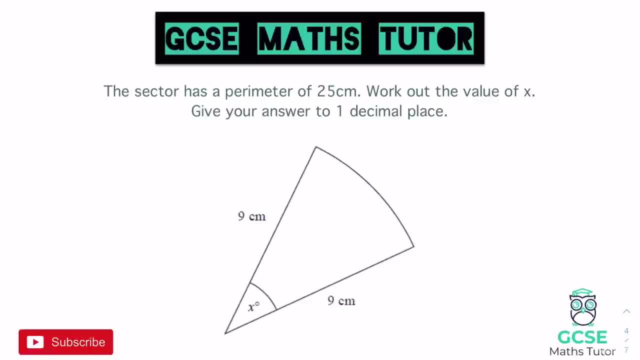 25. work out the value of x, and x is down there. it's the angle within the sector. then it says: give your answer to one decimal place. now, obviously, when it comes to this, it says that's the perimeter, there- 25. it doesn't say the arc length or anything like that. it says that's the perimeter and we've 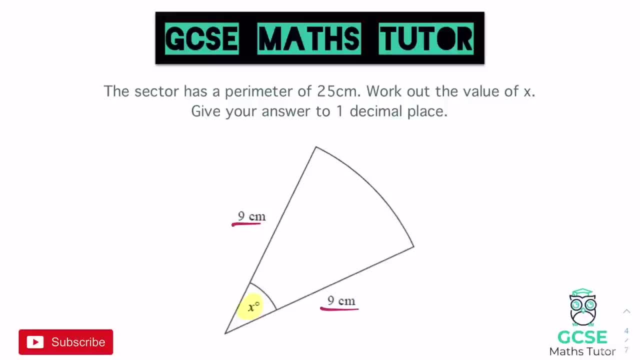 already got nine and nine around the perimeter there and that adds up to 18. so if we take that 25, so 25, take away 18, that leaves us with the remainder of seven there. so we've got seven centimetres for the arc length. now that's okay. that means, if we know the arc length, okay and we 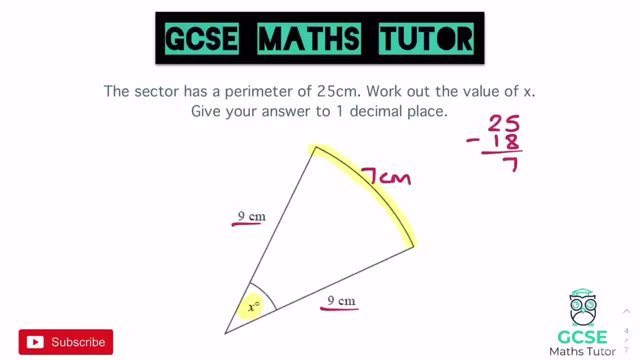 know the radius, then we can go about working out the angle there. because if we think about our formula for arc length, okay, it's the circumference, or the arc length is equal to pi times diameter, and then we times it by the fraction over 360. there we go. now we know the diameter and we know. 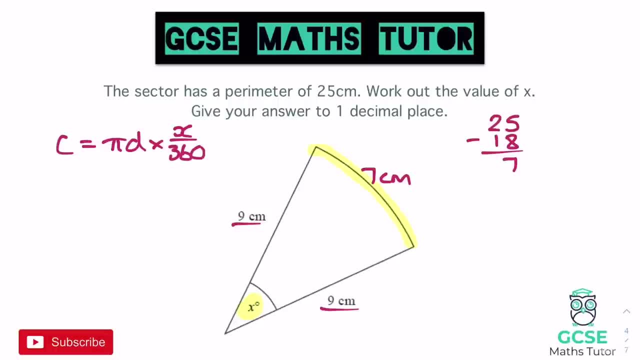 so actually the only thing we're missing is the angle. so actually, if I put all these pieces in, obviously we've got seven is the arc length, and that is going to be pi times the diameter, which is double the nine there, so 18, and let's write that down: d equals 18 and then that's multiplied. 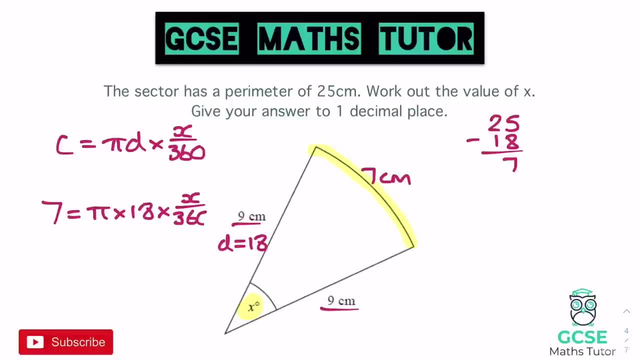 by x over 360. okay, so all we really need to do is figure out what number goes on top there to get us an answer of seven. now we could just guess numbers, we could put numbers into the calculator and just we could just go about rearranging this. now the first thing I can do to rearrange this is I can 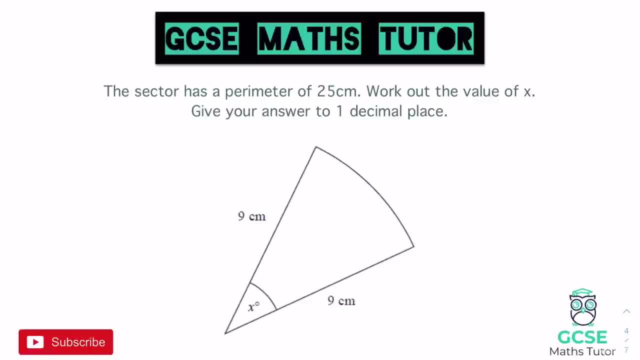 25. work out the value of x, and x is down there. it's the angle within the sector. then it says: give your answer to one decimal place. now, obviously, when it comes to this, it says that's the perimeter, there- 25. it doesn't say the arc length or anything like that. it says that's the perimeter and we've 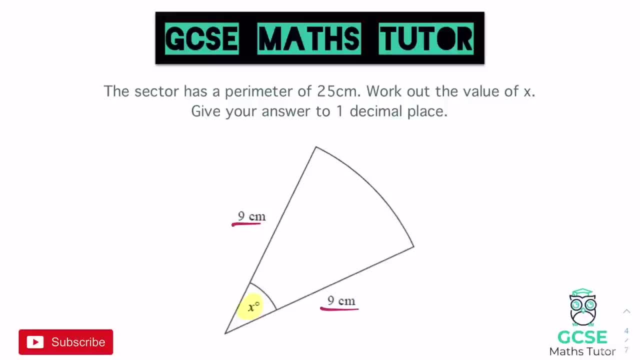 already got nine and nine around the perimeter there and that adds up to 18. so if we take that 25, so 25, take away 18, that leaves us with the remainder of seven there. so we've got seven centimetres for the arc length. now that's okay. that means, if we know the arc length, okay and we 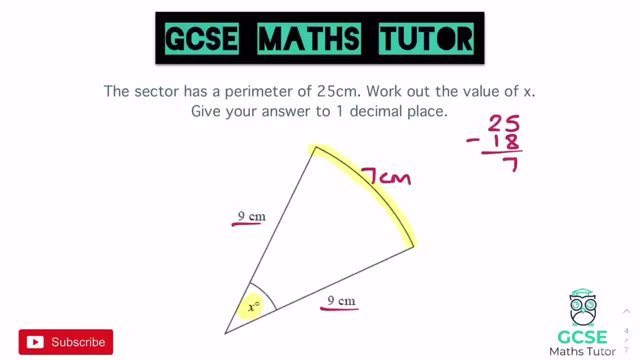 know the radius, then we can go about working out the angle there. because if we think about our formula for arc length, okay, it's the circumference, or the arc length is equal to pi times diameter, and then we times it by the fraction over 360. there we go. now we know the diameter and we know. 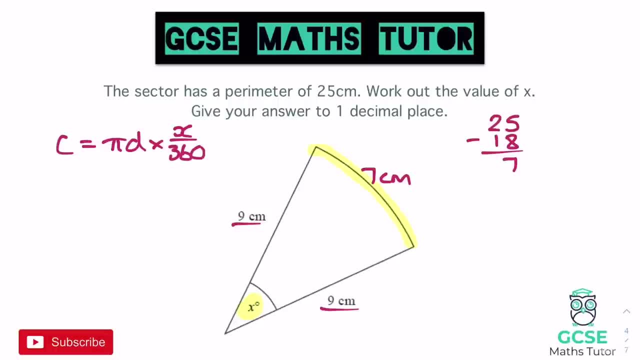 so actually the only thing we're missing is the angle. so actually, if I put all these pieces in, obviously we've got seven is the arc length, and that is going to be pi times the diameter, which is double the nine there, so 18, and let's write that down: d equals 18 and then that's multiplied. 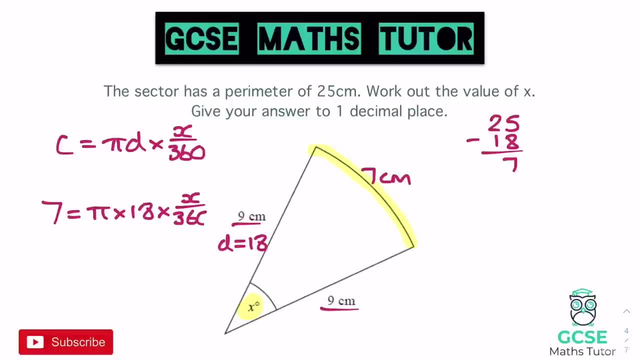 by x over 360. okay, so all we really need to do is figure out what number goes on top there to get us an answer of seven. now we could just guess numbers, we could put numbers into the calculator and just we could just go about rearranging this. now the first thing I can do to rearrange this is I can 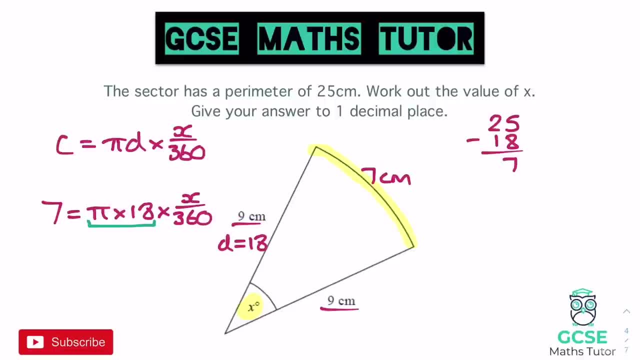 divide both sides by this 18 pi. again, I can just move that underneath the seven. okay, start dividing everything over. so let's just go about doing that. let's do seven divided by the 18 pi, okay, it's got to equal x over 360. there we go. so, if we go about working that out- because I can actually 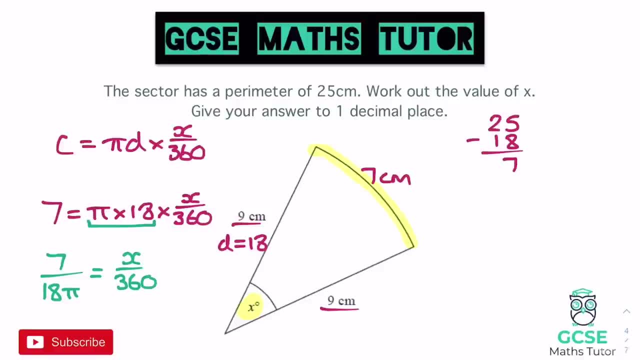 work out seven over 18 pi, seven divided by 18 pi, and that equals zero point one two. let's have a look, let's write this down over here. so we've got zero point one. two, three, seven, eight, seven and a few more decimals is equal to x divided by 360. 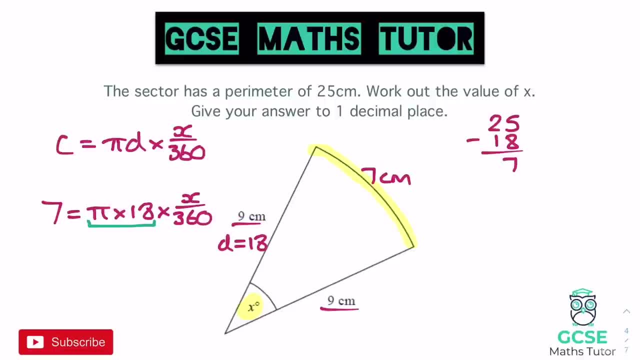 divide both sides by this 18 pi. again, I can just move that underneath the seven. okay, start dividing everything over. so let's just go about doing that. let's do seven divided by the 18 pi, okay, it's got to equal x over 360. there we go. so, if we go about working that out- because I can actually 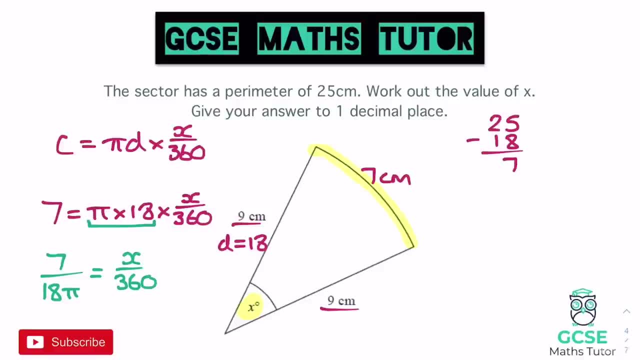 work out seven over 18 pi, seven divided by 18 pi, and that equals zero point one two. let's have a look, let's write this down over here. so we've got zero point one. two, three, seven, eight, seven and a few more decimals is equal to x divided by 360. 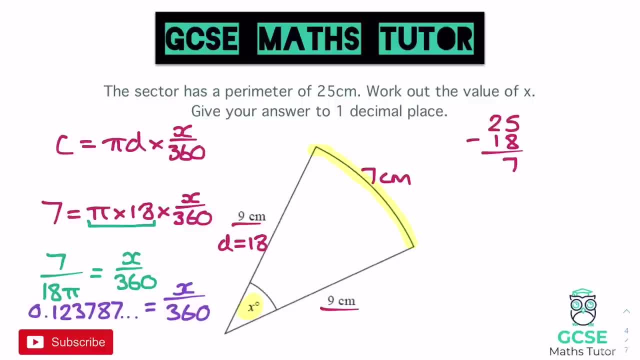 Now again, we've only got one little step now to finish this off, because obviously I don't want to know what x over 360 is. I want to know what x is. so if I just times both sides by 360 now to reverse that divide there, and so I'm just going to in my calculator: times 360. 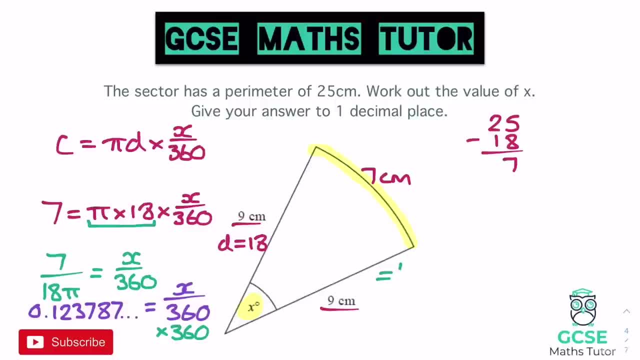 and it gives me my answer. there I get an answer and it comes out as 44.563. I'm going to stop there. it does keep on going, but we only want it to one decimal place. so obviously times it by 360 there gives us this answer. we want it to one decimal place, so chop it after the five and let's have. 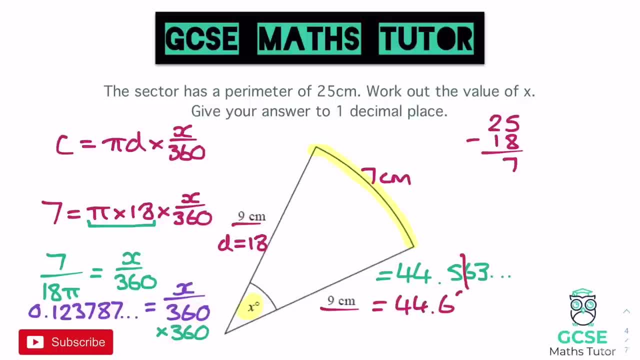 a look, we have 44 point and that is going to round up to six there. so 44.6 degrees is our final answer. there we go. a nice little thing. you can always go back and check. you can put 44 point, what is it? 44.6. 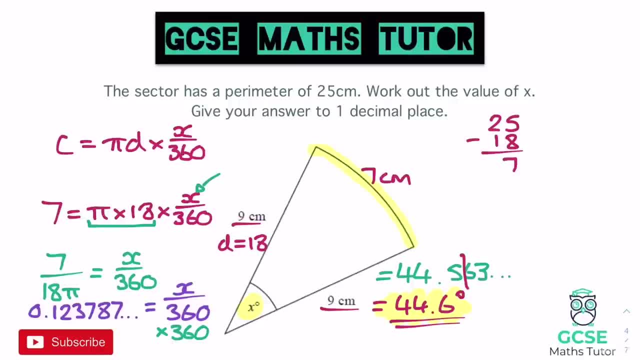 degrees in place of x here and just make sure that you do get seven. obviously we've got our answer rounded there. so it's not going to be exactly seven unless we use that full number on our calculator there. but you can always go back and check just to make sure that you've rearranged. 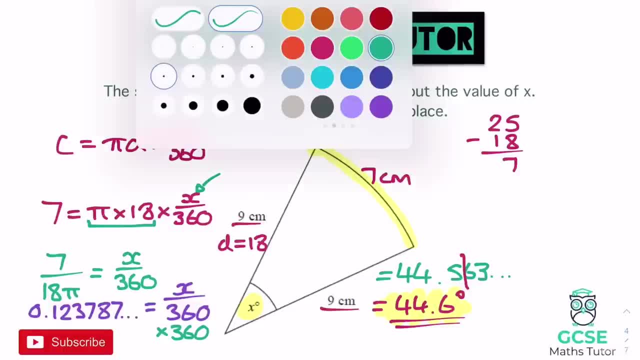 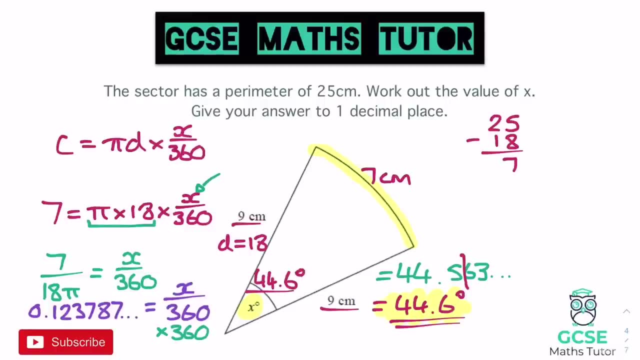 it correctly. okay, so once you've got that angle, obviously there's a few different things that you can now be asked to do. let's have a look: 44.6 degrees. we could actually now be asked to work out the area. now it doesn't in this question, but I'm just thinking about, obviously, the progression. 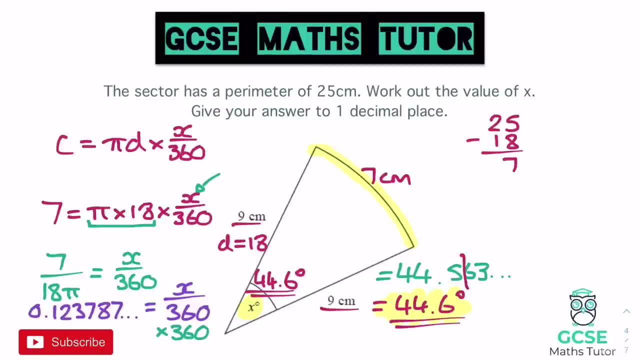 of this topic and where it could go. you could actually now just be asked to work out the area. so if we were asked to do that, we would now just do pi r squared multiplied by 44.6 over 360- okay, just plugging it into that formula that we did before, and likewise that could be done in reverse. 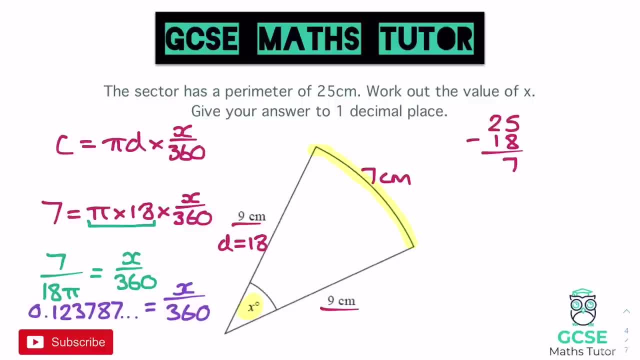 Now again, we've only got one little step now to finish this off, because obviously I don't want to know what x over 360 is. I want to know what x is. so if I just times both sides by 360 now to reverse that divide there, and so I'm just going to in my calculator: times 360. 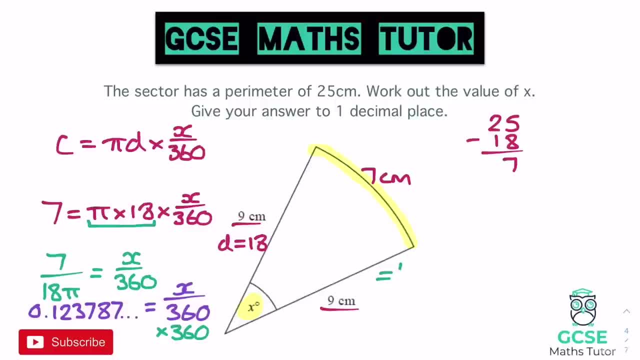 and it gives me my answer. there I get an answer and it comes out as 44.563. I'm going to stop there. it does keep on going, but we only want it to one decimal place. so obviously times it by 360 there gives us this answer. we want it to one decimal place, so chop it after the five and let's have. 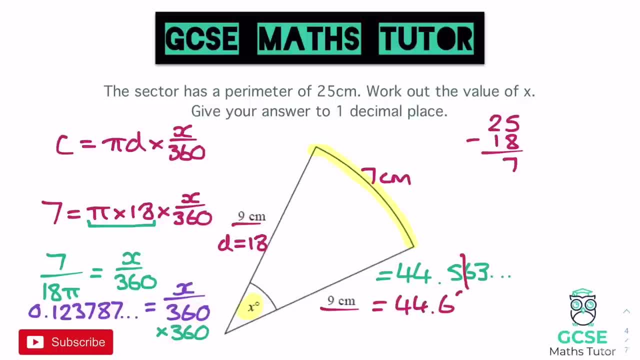 a look, we have 44 point and that is going to round up to six there. so 44.6 degrees is our final answer. there we go. a nice little thing. you can always go back and check. you can put 44 point, what is it? 44.6. 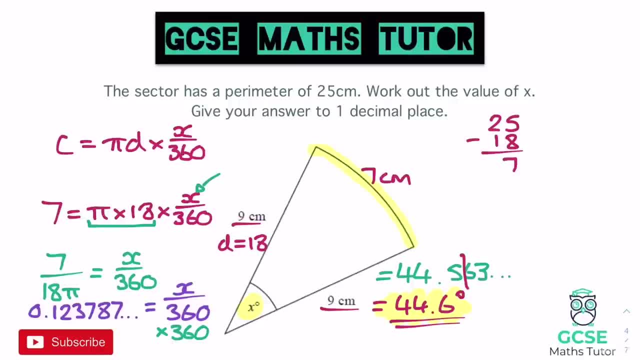 degrees in place of x here and just make sure that you do get seven. obviously we've got our answer rounded there. so it's not going to be exactly seven unless we use that full number on our calculator there. but you can always go back and check just to make sure that you've rearranged. 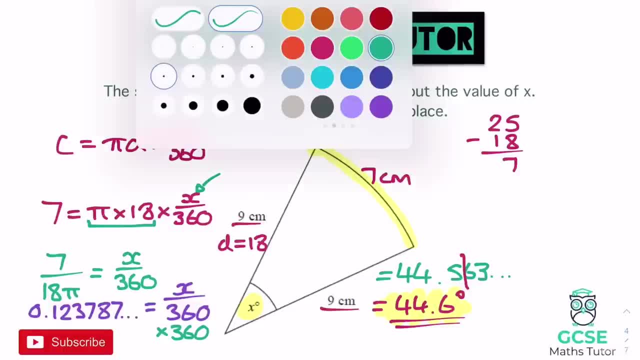 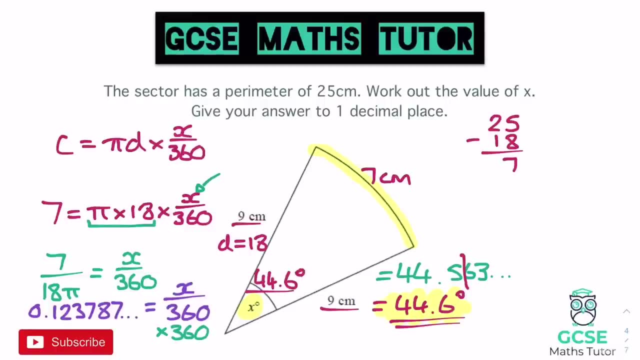 it correctly. okay, so once you've got that angle, obviously there's a few different things that you can now be asked to do. let's have a look: 44.6 degrees. we could actually now be asked to work out the area. now it doesn't in this question, but I'm just thinking about, obviously, the progression. 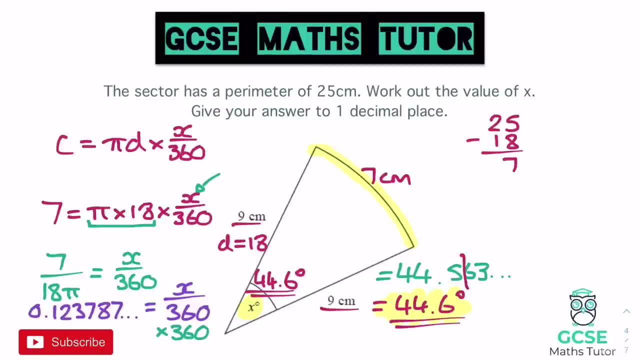 of this topic and where it could go. you could actually now just be asked to work out the area. so if we were asked to do that, we would now just do pi r squared multiplied by 44.6 over 360- okay, just plugging it into that formula that we did before, and likewise that could be done in reverse. 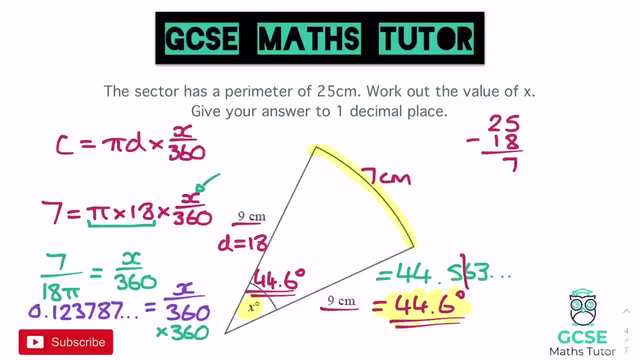 as well. we could have been given the area to work out the angle and then look at working out the arc length from that once we've got that angle. okay, so just a little bit in reverse, obviously talking about perimeter, talking about arc length and then actually potentially asking you to work out the 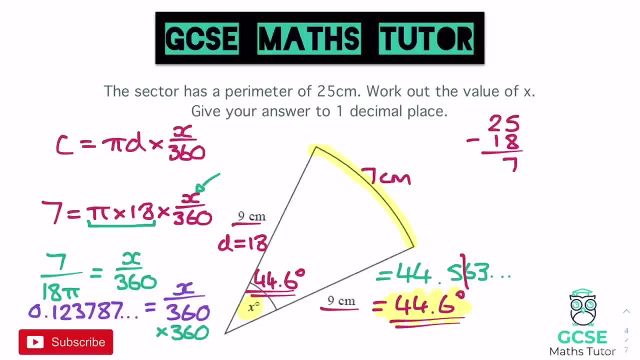 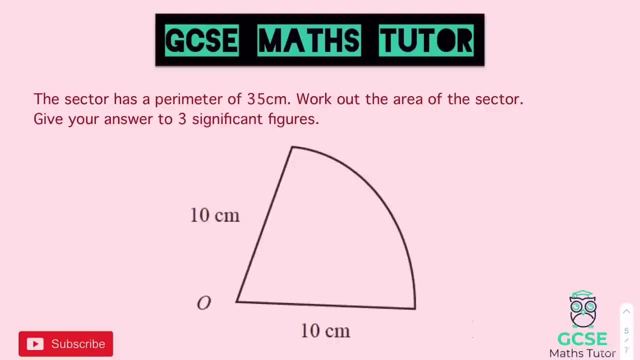 area, and that's something you're going to have a go at now on a very similar question to this. so let's have a look at that one, okay, so the structure of this equation is going to be very similar to the one that we just looked at. we've got a sector. it tells us the perimeter. 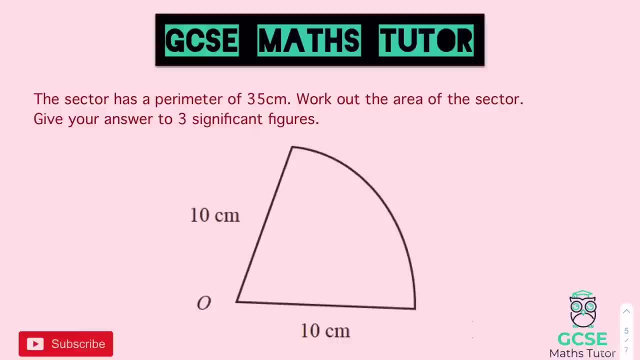 and it asks you to work out the area. so you need to go about working out that angle within the sector and then using that to work out the area. so pause the video there. have a go and we'll go over the answer in a sec. okay, so it says the perimeter is 35. so we have 10 and 10 at the 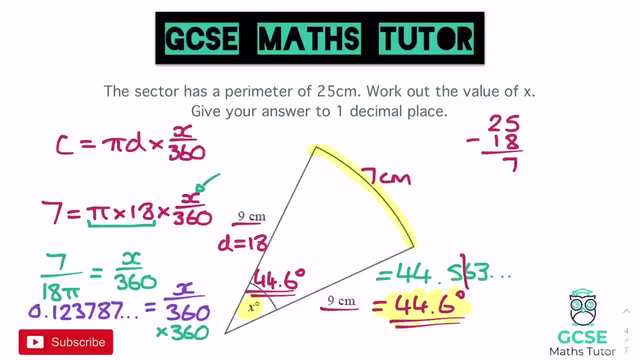 as well. we could have been given the area to work out the angle and then look at working out the arc length from that once we've got that angle. okay, so just a little bit in reverse, obviously talking about perimeter, talking about arc length and then actually potentially asking you to work out the 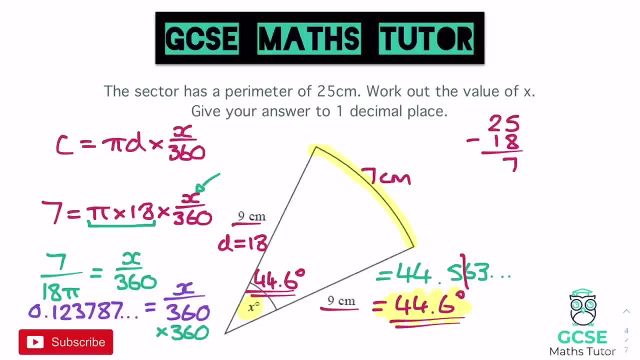 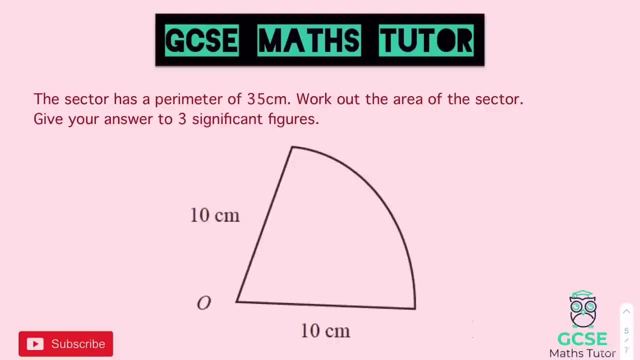 area, and that's something you're going to have a go at now on a very similar question to this. so let's have a look at that one, okay, so the structure of this equation is going to be very similar to the one that we just looked at. we've got a sector. it tells us the perimeter. 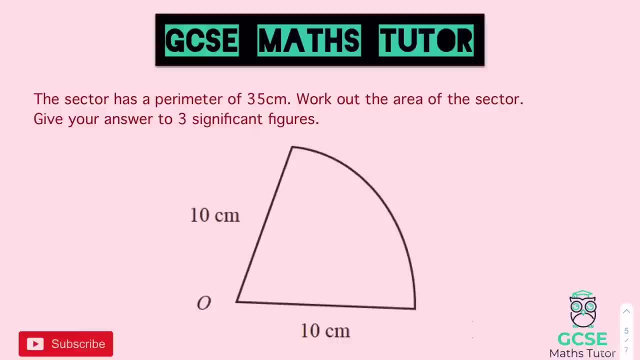 and it asks you to work out the area. so you need to go about working out that angle within the sector and then using that to work out the area. so pause the video there. have a go and we'll go over the answer in a sec. okay, so it says the perimeter is 35. so we have 10 and 10 at the 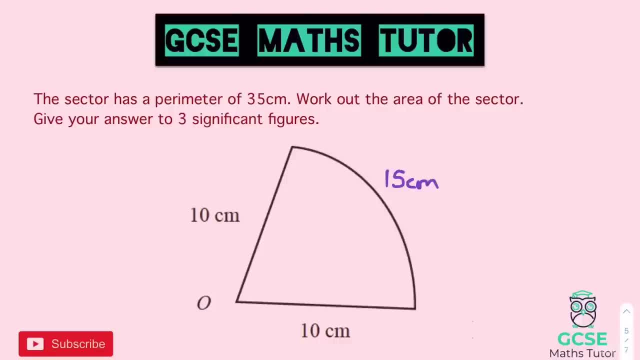 moment and that gives us 15 left over to make sure that that has a perimeter of 35 there. so we know that the arc length is 15. we just want to work out what this angle is here, this x degrees. so if we plug all these pieces into our formula again, we've got that, the arc. 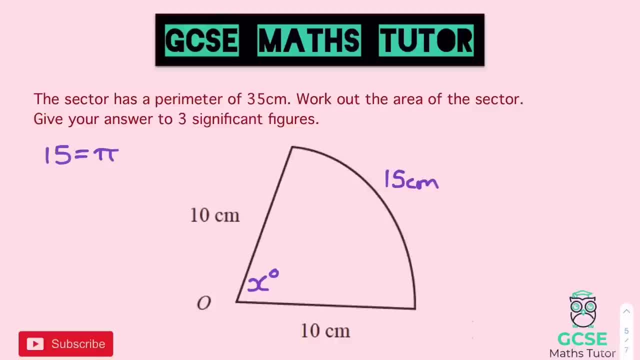 length, 15 has to equal pi times the diameter, and again the diameter is double the radius, so 20. so pi times 20 times x over 360. whatever that is, there we go, and if we go about rearranging that, let's have a look. we've got 15 divided by this pi times 20, so divided by the 20 pi. 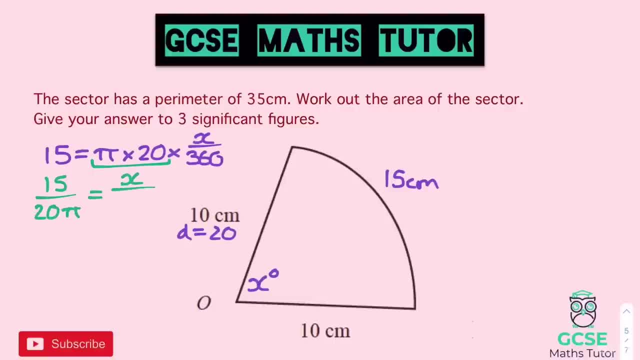 and then it's going to equal x over 360.. There we go on to the next step. let's work out 15 divided by 20 pi, and that comes out as 0.238. there we go. so 0.238- I'm going to leave that on my calculator- is equal to this x over 360. 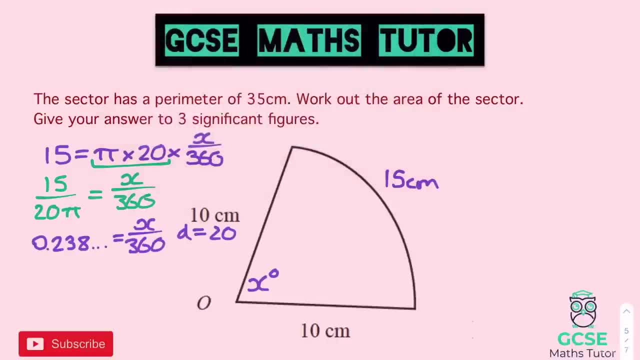 and again. multiplying both sides by 360 now to get the size of our angle. so times by 360 and let's see what we get for x. there we go and we get 85.943. so 85.943 and a little few more decimals, we've got 66927. I'm going to write it all down because 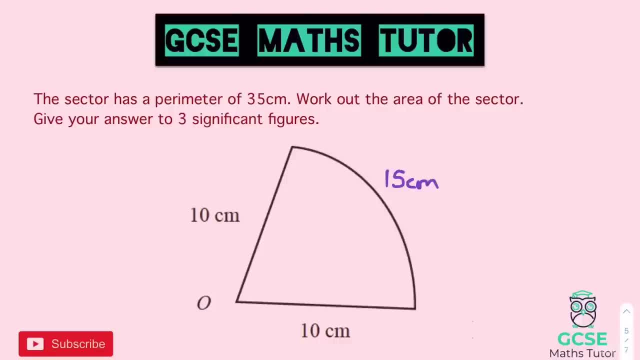 moment and that gives us 15 left over to make sure that that has a perimeter of 35 there. so we know that the arc length is 15. we just want to work out what this angle is here, this x degrees. so if we plug all these pieces into our formula again, we've got that, the arc. 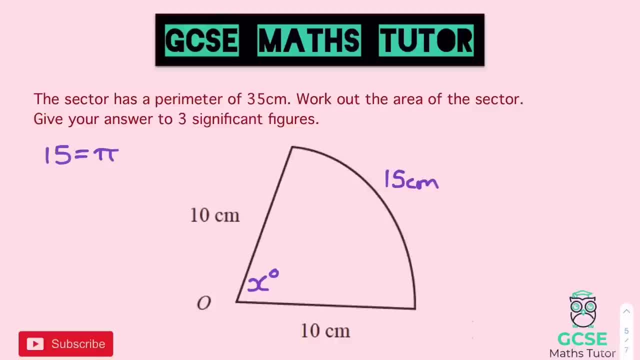 length, 15 has to equal pi times the diameter, and again the diameter is double the radius, so 20. so pi times 20 times x over 360. whatever that is, there we go, and if we go about rearranging that, let's have a look. we've got 15 divided by this pi times 20, so divided by the 20 pi. 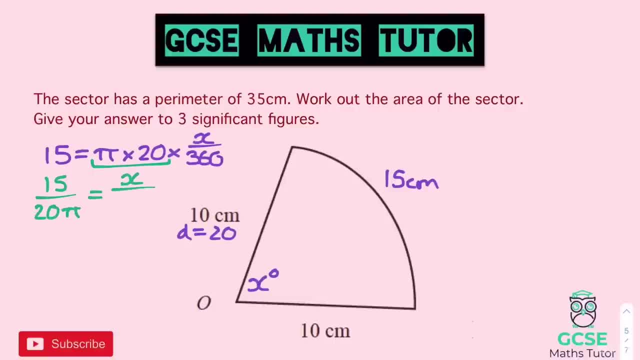 and then it's going to equal x over 360.. There we go on to the next step. let's work out 15 divided by 20 pi, and that comes out as 0.238. there we go. so 0.238- I'm going to leave that on my calculator- is equal to this x over 360. 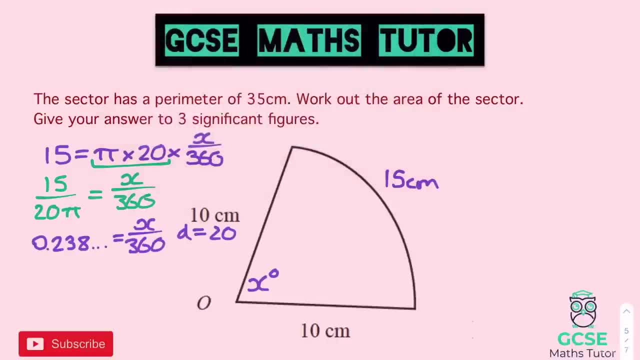 and again. multiplying both sides by 360 now to get the size of our angle. so times by 360 and let's see what we get for x. there we go and we get 85.943. so 85.943 and a little few more decimals, we've got 66927. I'm going to write it all down because 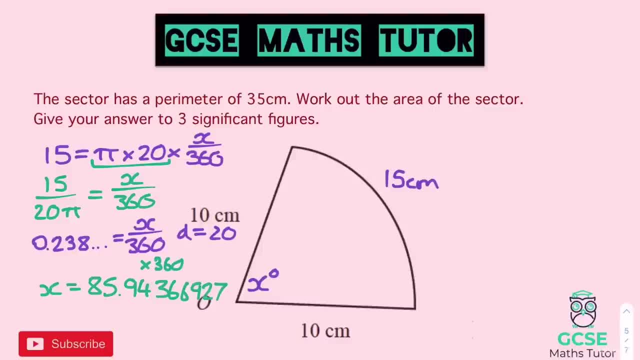 we're not quite finished yet. so now we've got the angle. okay, I'm just going to write that in here. so we've got 85.9 degrees. okay, obviously that's rounded to three significant figures, but I'm going to use the full answer to work out the next step, because now it wants us to work out the area. 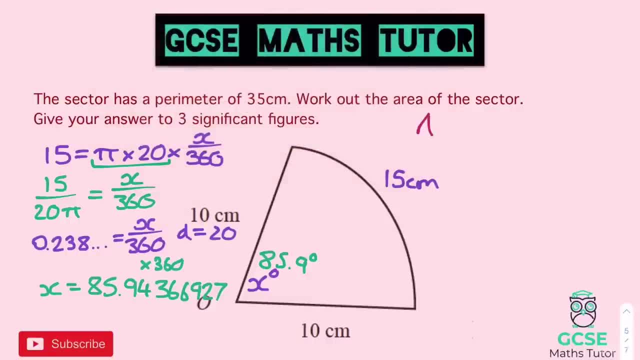 so obviously, the formula for our area. let's have a look. we've got the area equals pi r squared times the angle over 360. in this case that'll be 85.9 over 360. there we go. so in my calculator I'm going to type this all in, I'm going to do the to get work out the area. I'm going to do pi times 10. 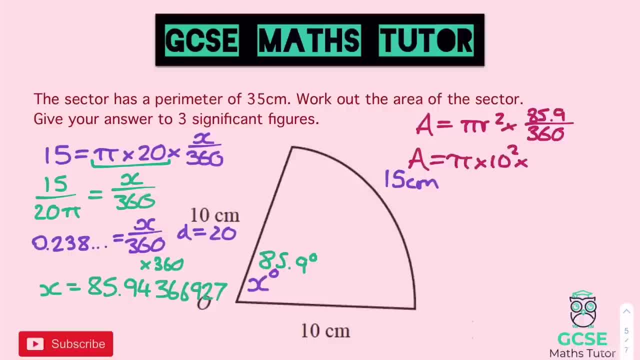 squared, the radius squared and then times by this: 85.9 over 360. I'm going to use the answer in my calculator so I've still got that full number there and I'm not going to get any rounding errors. so we've got pi times, 10 squared times and then open my fraction answer over 360. 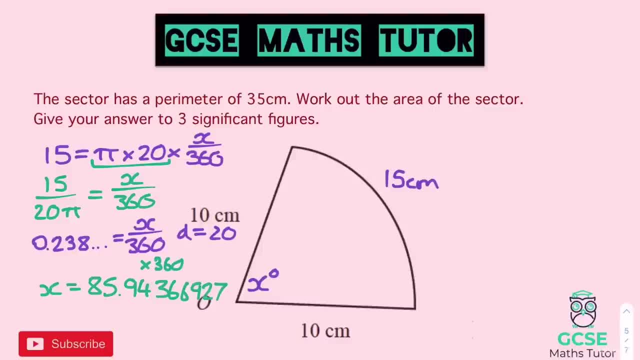 we're not quite finished yet. so now we've got the angle. okay, I'm just going to write that in here. so we've got 85.9 degrees. okay, obviously that's rounded to three significant figures, but I'm going to use the full answer to work out the next step, because now it wants us to work out the area. 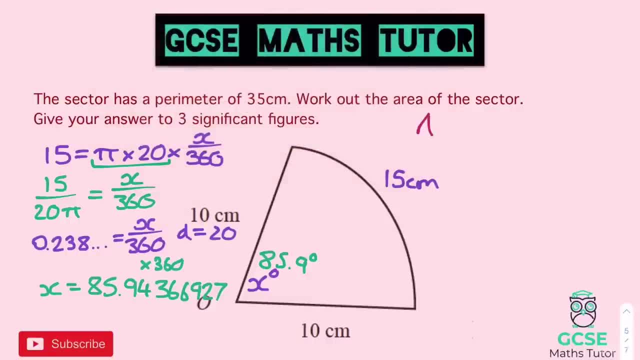 so obviously, the formula for our area. let's have a look. we've got the area equals pi r squared times the angle over 360. in this case that'll be 85.9 over 360. there we go. so in my calculator I'm going to type this all in, I'm going to do the to get work out the area. I'm going to do pi times 10. 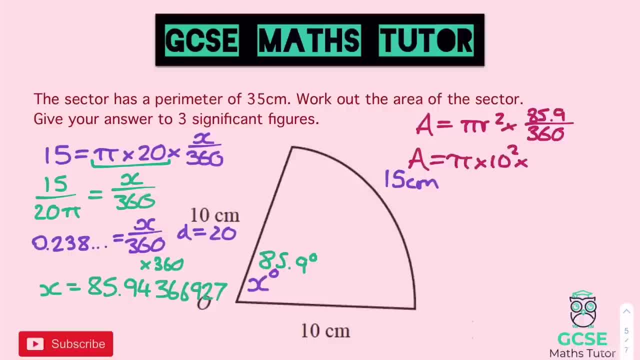 squared, the radius squared and then times by this: 85.9 over 360. I'm going to use the answer in my calculator so I've still got that full number there and I'm not going to get any rounding errors. so we've got pi times, 10 squared times and then open my fraction answer over 360. 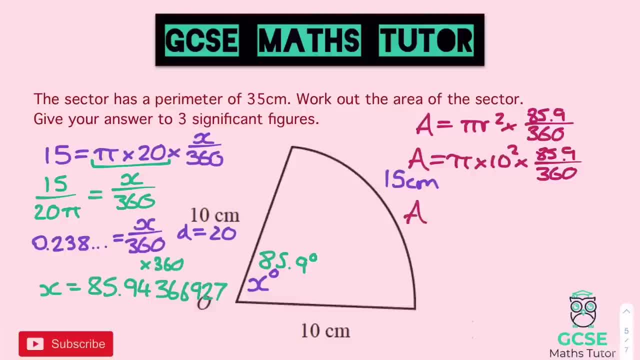 there we go and we get the answer 75. perfect, that comes out as 75, exactly right, there we go. that's a bit of a strange one where it comes out as exactly 75, but in in the terms of this question, let's have a think about how we would write that to three significant figures, because at the moment, 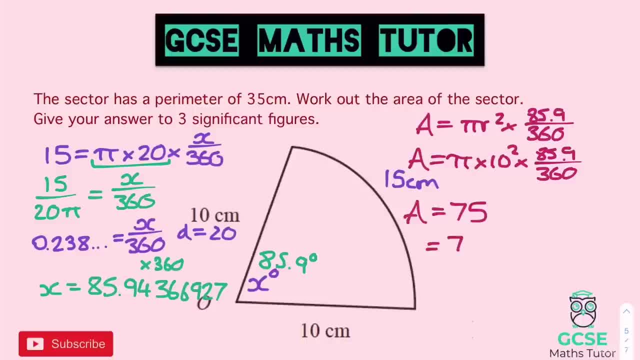 that's only two significant figures there, so we would have to write 75.0. there we go, and that is an area, so that is centimeters squared. there we go, and there's our final answer. a little bit strange to be asked to write that into the formula. so we're going to have to write that into the formula. 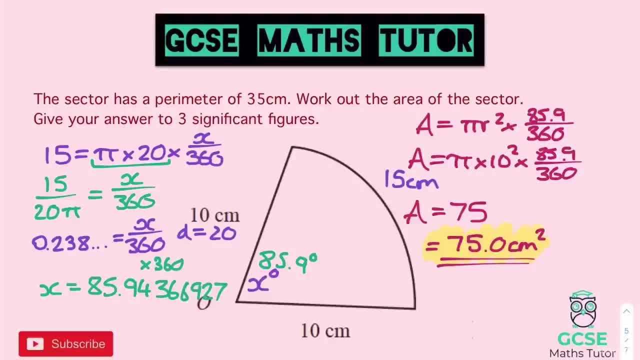 three significant figures. but if that situation does occur and you have to put a zero on the end to ensure that it's three significant figures, then we'll absolutely do so there. okay, but there we go. that's how you go about doing this question. now we've got one more question to have a look at. 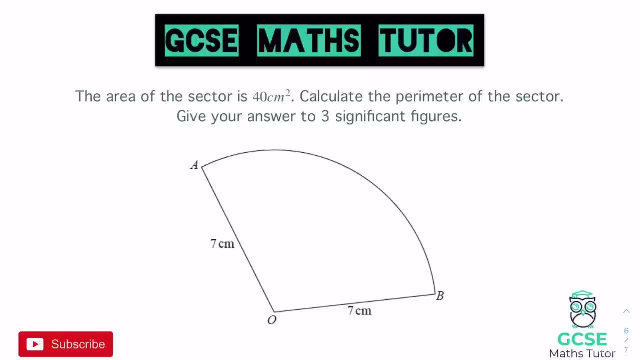 before we finish. so here that is okay. so this question here is almost the reverse of what we just did. okay, in this question you're given the area of the sector and you're asked to work out the perimeter. so essentially it's asking you to work out the arc length and then establish what. 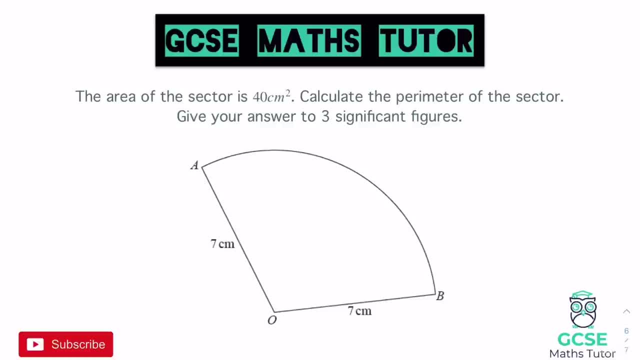 the perimeter is once you've got that. so it's quite a lot of working out to do here, but nothing really different to what we've just done. so we're going to have to work out the perimeter we've just looked at, obviously just starting with the area rather than the arc length. so have a go. 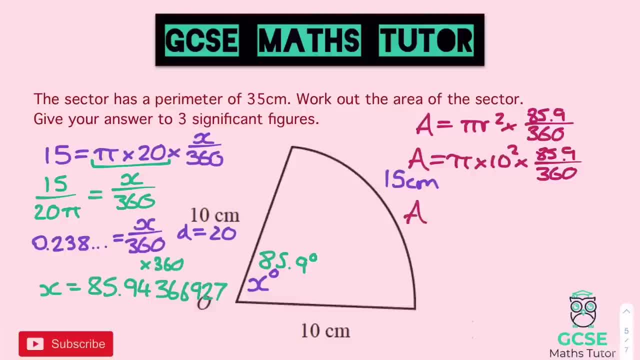 there we go and we get the answer 75. perfect, that comes out as 75, exactly right, there we go. that's a bit of a strange one where it comes out as exactly 75, but in in the terms of this question, let's have a think about how we would write that to three significant figures, because at the moment, 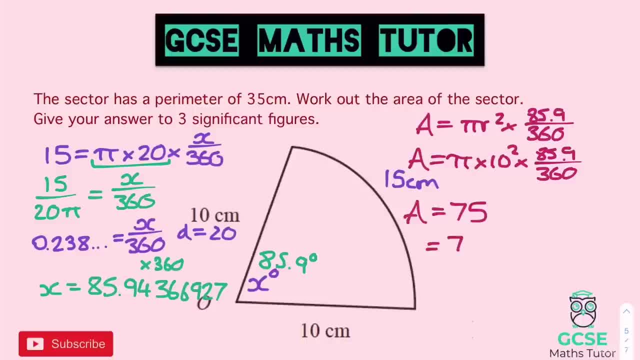 that's only two significant figures there, so we would have to write 75.0. there we go, and that is an area, so that is centimeters squared. there we go, and there's our final answer. a little bit strange to be asked to write that into the formula. so we're going to have to write that into the formula. 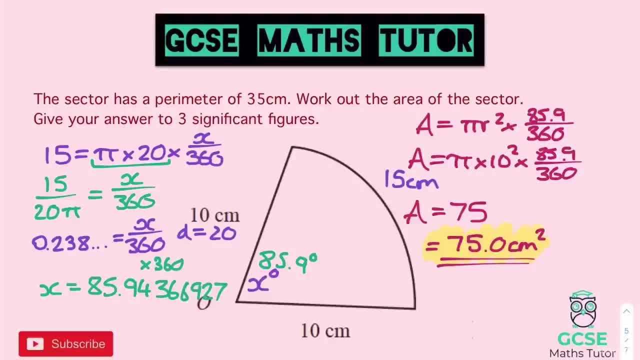 three significant figures. but if that situation does occur and you have to put a zero on the end to ensure that it's three significant figures, then we'll absolutely do so there. okay, but there we go. that's how you go about doing this question. now we've got one more question to have a look at. 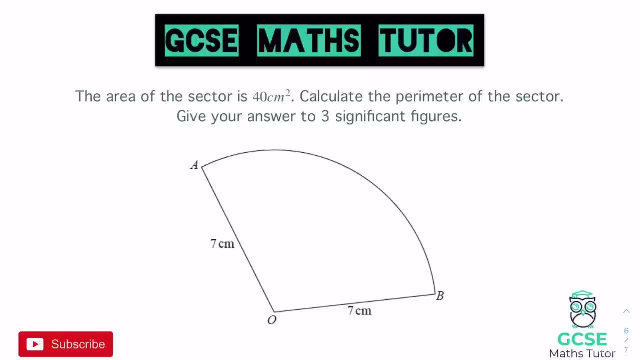 before we finish. so here that is okay. so this question here is almost the reverse of what we just did. okay, in this question you're given the area of the sector and you're asked to work out the perimeter. so essentially it's asking you to work out the arc length and then establish what. 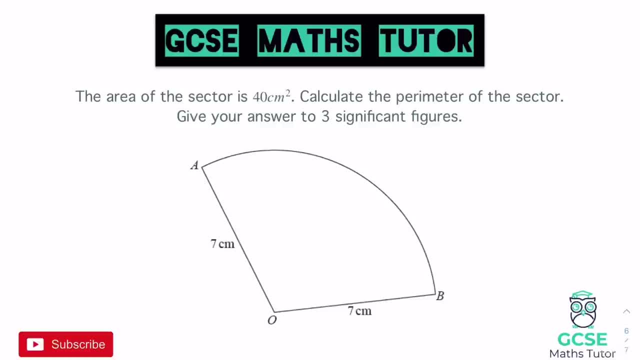 the perimeter is once you've got that. so it's quite a lot of working out to do here, but nothing really different to what we've just done. so we're going to have to work out the perimeter we've just looked at, obviously just starting with the area rather than the arc length. so have a go. 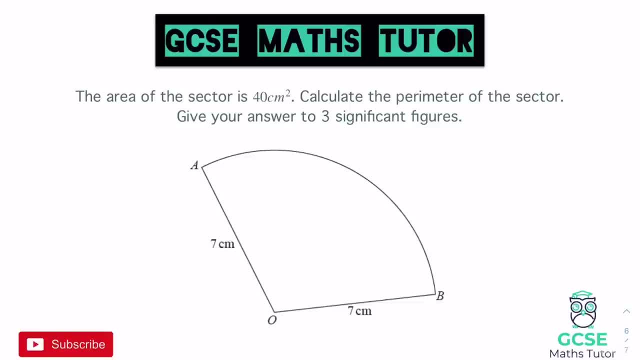 at this question. pause video there. see what you get. it's our last one and then we'll go over the answer in a sec. okay, so for this one we've got the area is 40.. so our area formula is pi r squared. so we have: 40 is equal to pi r squared. so pi times 7, squared times the angle over 360, and again. 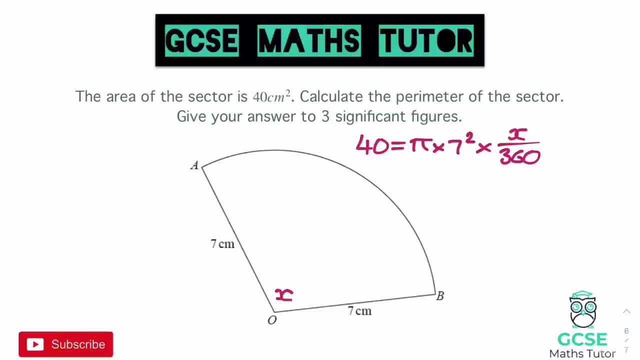 we don't know the angle, so we're going to work that out and let's label that down here as x. so let's rearrange that. so we want to get rid of the pi times 7 squared, so we'll put that underneath the 40 we'll divide. 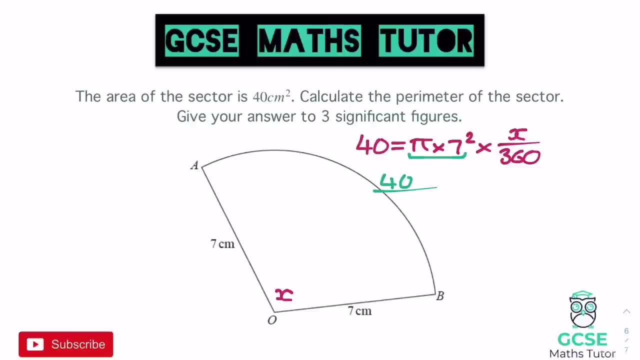 both sides by that. so we've got 40 divided by 7 squared is 49, so we'll put 49 pi just to save writing that down, and that's going to equal the x over 360.. there we go, so 40 divided by 49 pi. 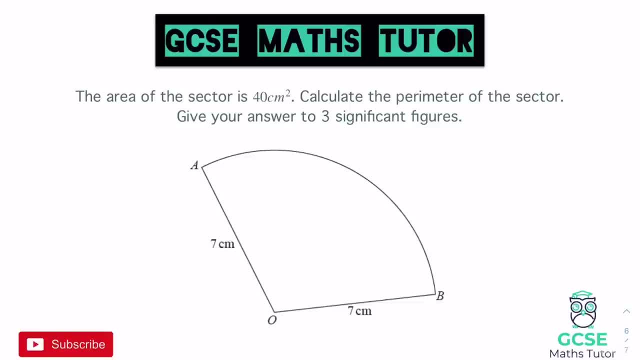 at this question. pause video there. see what you get. it's our last one and then we'll go over the answer in a sec. okay, so for this one we've got the area is 40, so our area formula is pi r squared. so we have: 40 is equal to pi r squared. so pi times seven, squared times the angle over 360, and again. 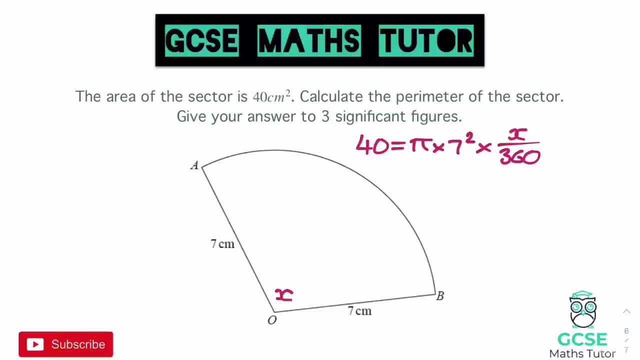 we don't know the angle, so we're going to work that out and let's label that down here as x. so let's rearrange that. so we want to get rid of the pi times 7 squared, so we'll put that underneath the 40 we'll divide. 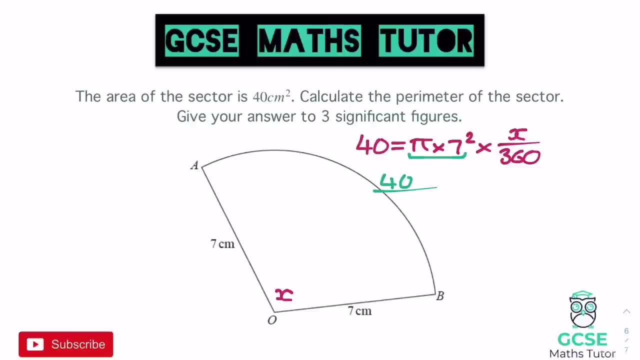 both sides by that. so we've got 40 divided by 7 squared is 49, so we'll put 49 pi just to save writing that down, and that's going to equal the x over 360.. there we go, so 40 divided by 49 pi. 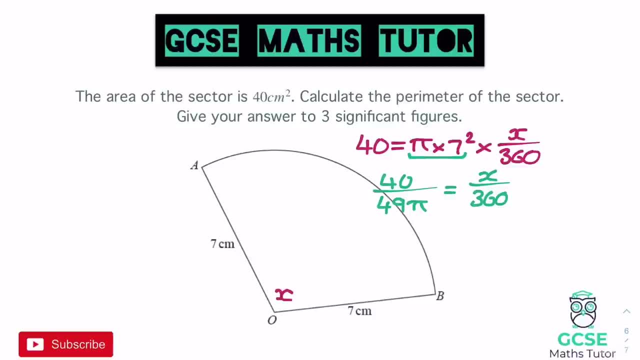 comes out as 0.259. let's have a look. so 0.259 and a few more decimals, is x over, equals x over 360, and so we'll times by 360 again to get the size of our angle. there we go. so times 360 on the calculator, and there we go, we get 90. so we'll look. 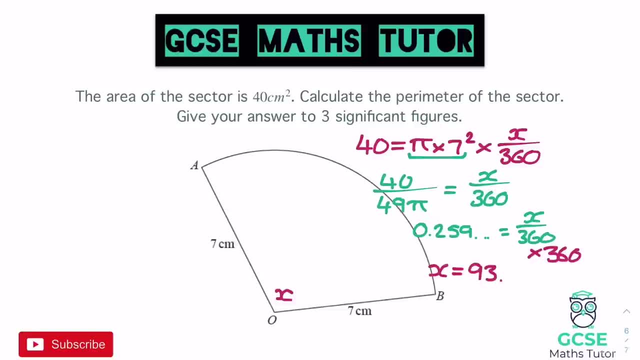 93.544, and again a few more decimals. I'm going to leave it on my calculator for the moment. there we are. that's 93.544 degrees. okay, so we've got the size of the angle, and now we can use that to work out the length of the arc. 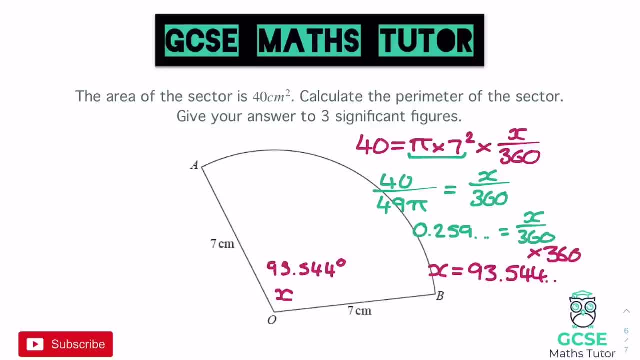 okay, so obviously circumference is pi times diameter. so we're going to work this out. we're going to do pi times the diameter. let's have a look. so the diameter is double the radius, so 14.. so pi times 14, multiplied by this, 93.544 over 360. 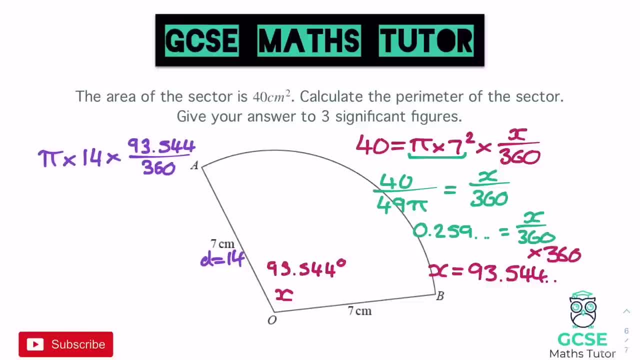 there we go. that's going to give us the length of the arc, and again, I'm going to use the answer button in my calculator. so pi times 14, times answer over 360, and that gives me a nice decimal here. here we go: 11.428571. 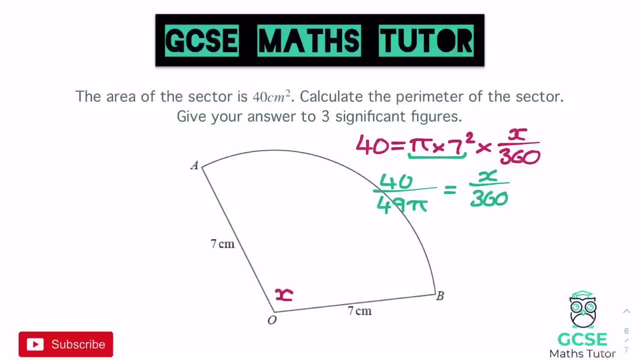 comes out as 0.259. let's have a look. so 0.259 and a few more decimals, is x over, equals x over 360, and so we'll times by 360 again to get the size of our angle. there we go. so times 360 on the calculator, and there we go, we get 90. so we'll 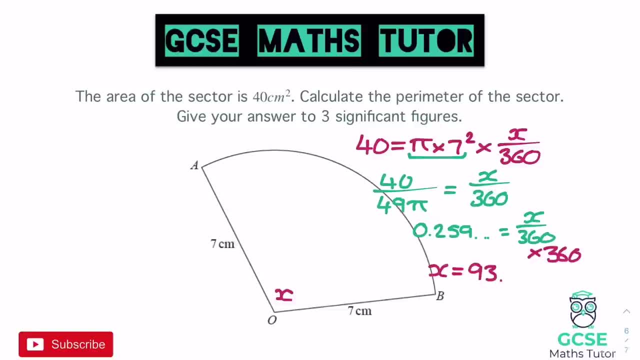 look, 93.544, and again a few more decimals. i'm going to leave it on my calculator for the moment. there we are. that's 93.544 degrees. okay, so we've got the size of the angle, and now we can use that to work out the length of the arc. 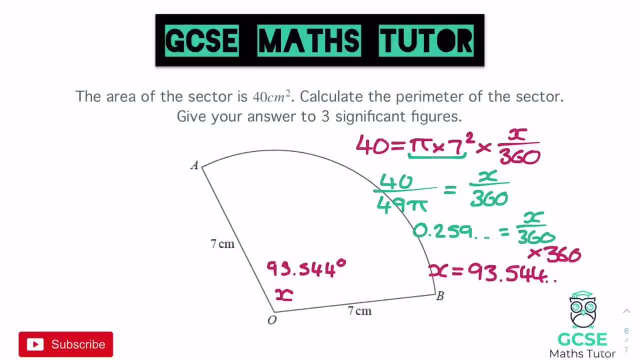 okay, so obviously circumference is pi times diameter. so we're going to work this out. we're going to do pi times the diameter. let's have a look. so the diameter is double the radius, so 14.. so pi times 14, multiplied by this, 93.544 over 360. 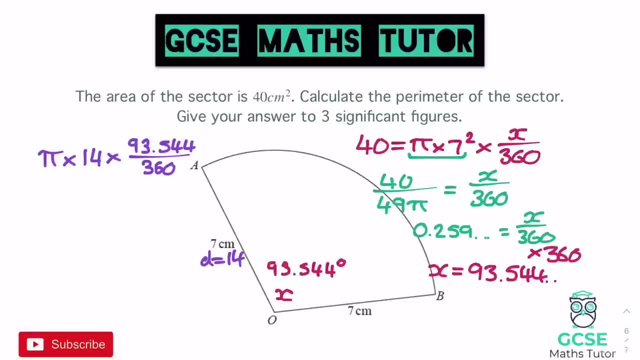 there we go. that's going to give us the length of the arc, and again, I'm going to use the answer button in my calculator. so pi times 14, times answer over 360, and that gives me a nice decimal here. here we go: 11.428571. 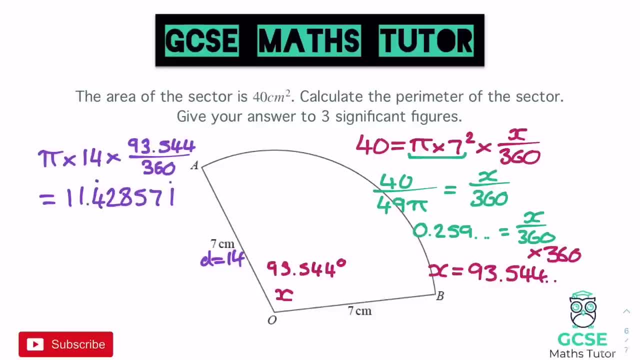 and a recurring decimal there above the four and the one. okay, so there's our answer for the length of the arc. now once my answer to three significant figures and both my radiuses. there are seven centimeters, so I'm going to round this to three significant figures now and then think about what. 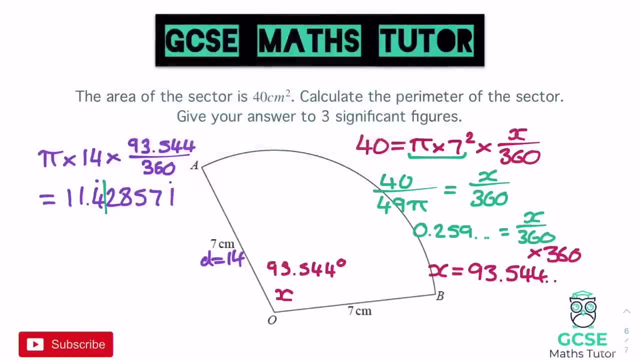 I can do from there. so one, one, four, so it's after the four, so that's going to round to four and then 11.4. okay, and obviously the units here are centimeters and that's the length of my arc there. so if we label that on the diagram, the length of the arc is 11.4 and it wants the perimeter. so 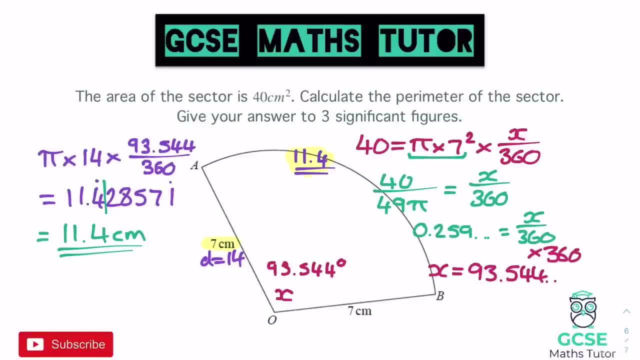 the perimeter. we're going to have to take this one, I'm going to have to take this one, I'm going to have to take this one, and we just need to add all of those together. so let's write that down: 11.4 plus 7 plus 7. and if we add those all up, let's have a look. what do we get? we get 25.4 there. we